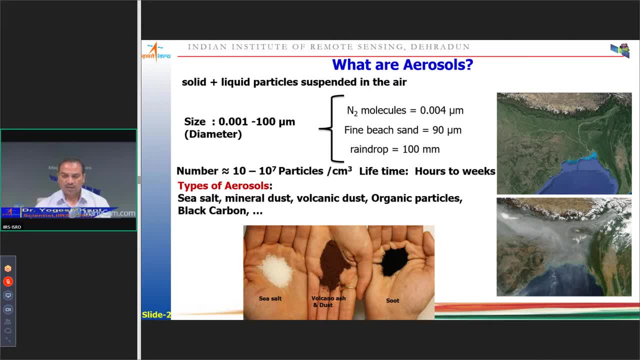 of the aerosols are particularly the dust and the volcano and the sea salt and types of aerosols. The picture shows the different kinds of the sizes of the different aerosol, as you see that the sea salt, the volcanic dust and the soot, the black carbon, These aerosols are variable. 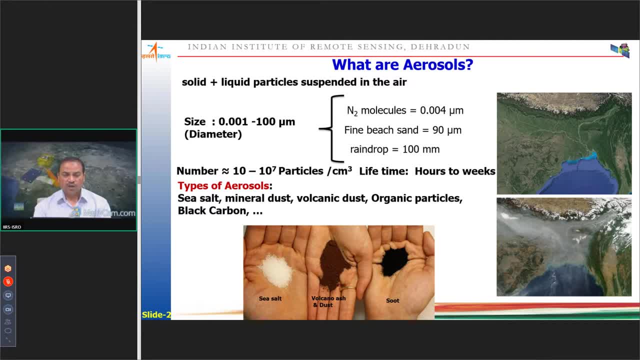 in nature and also in different lifetimes, And though these planets are different, the iris holes are also multiple. You have to use a семьlet or a elliptical aperture, or that is a smaller aperture, to be able to go correctly. So here's a very small example. you can see, here we are the most important one of the. 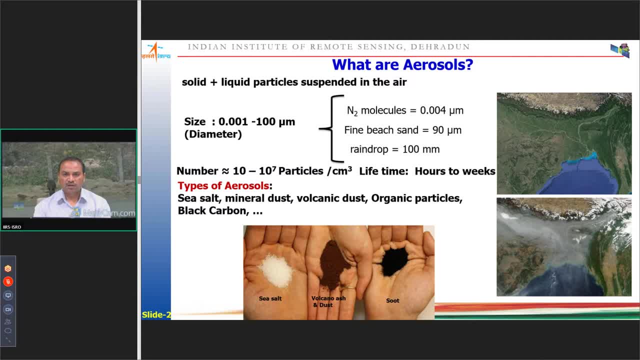 two. the most important is the celestial field, And you can see here that it's a large surface And this is the big one which is called the Theta, the vector position, and they come down to the surface also. the aerosols, they have much influence, they influence the radiation budget, that is, the Sun, Earth. 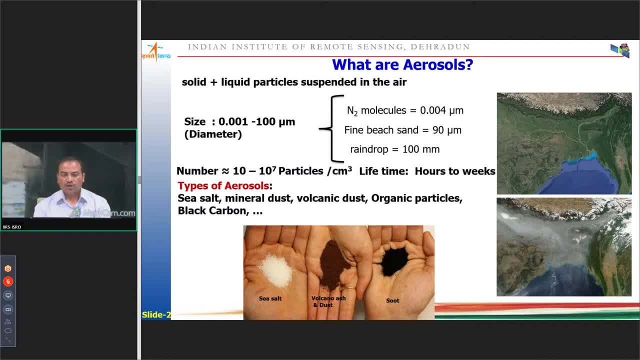 atmosphere budget and also it has they. they are responsible for the scattering, that is the absorption. the absorption that is warming, warming and then the cooling by scattering. also they, they have there. they are responsible for formation of the fog, the mist, the visibility effects, also the the cloud. 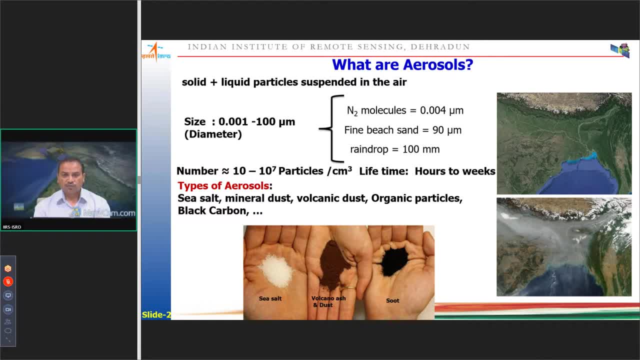 formation, because they are responsible for the cloud condensation nuclei and they become seeds for formation of clouds. and more cloud space, more backflow, cool, which means the light, the light in which the shade and the traveling scattering, so less amount of solar radiation reaching on the earth. so there 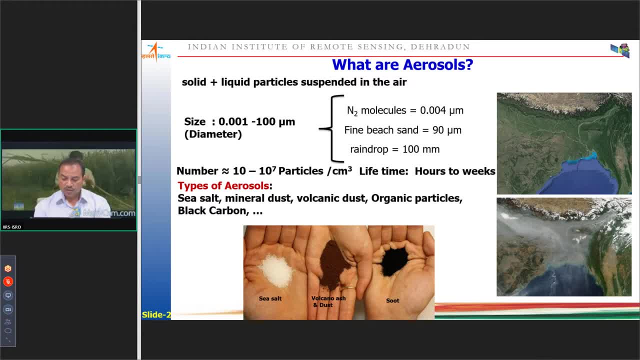 is a change of the earth radiation budget. also. the absorbing nature is warming. nature also attributes or adds to the greenhouse effect, which is creating a lot of warming and other effects in the earth radiation budget. when we talk about the satellite data, so they also affect the satellite data by 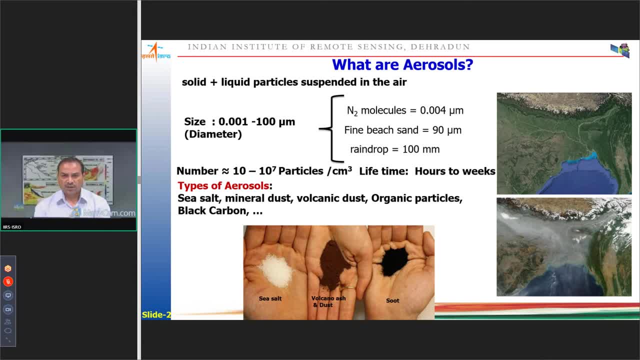 scattering the electronic radiation, so the signal, the deformation of the signal reaching the sensor. so we need to have an atmospheric corrections before we use four different applications. so the these are the main effects of the aerosol which we observe, of the aerosol which we observe, of the aerosol which we observe. 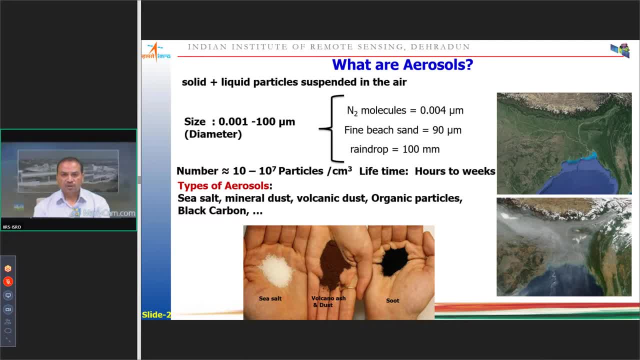 day-to-day events In the particular slide, if you see the two images, one in the upper right which you see that the eastern Indo-Gangetic plain of Bay of Bengal and the down one bottom one, due to the winter season, So there is a thick. 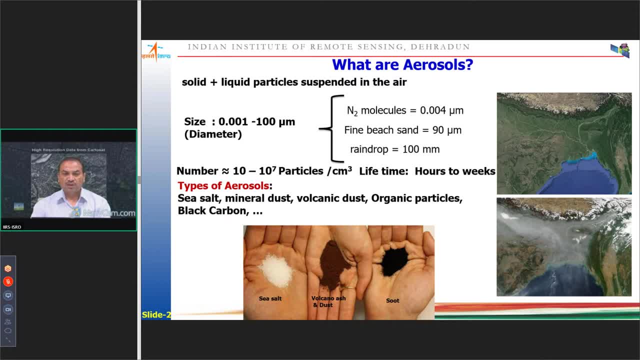 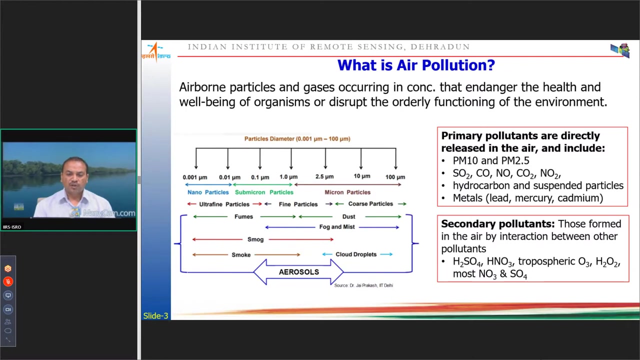 fog which is experiencing in the winter season, particularly over this area. So all this formation is due to the aerosols and then they settle down and they form as a seed and they affect a lot many perturbations Now coming about, the air pollution. Now, what is air pollution? The airborne particles. 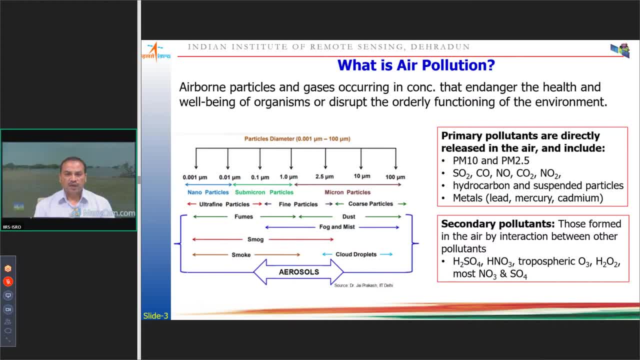 or the gases occurring in concentration that endanger the health and well-being of organisms, Whether it is human, animal, vegetation, wildlife or any material. The air, the air pollution also affects the materials, like we have the heritage sites, the monuments, and it affects that. 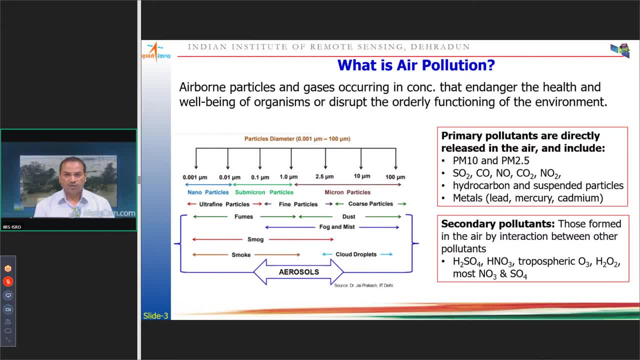 So, and also it disrupts the orderly function of the environment and the substances which which affect these. these substances are known as the air pollutants. So there are different particles or different substances that are above the the common range, that is, the standard range, and then it becomes dangerous. and then, if we identify 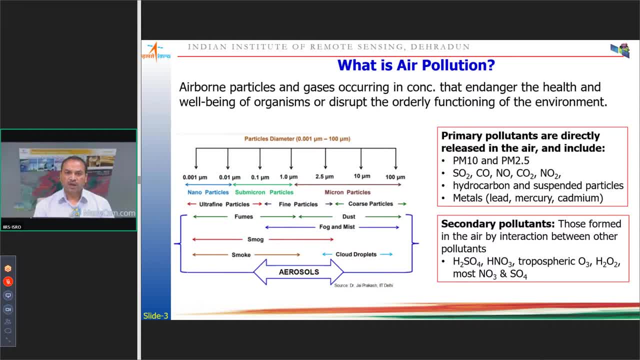 pollutants and then we try to analyze what are the chemical reactions and what are the effects on the well-being of different organisms. These air pollutants are of two types. one is the primary pollutants and secondary pollutants. AboutATAC, military learned research should be done by some higher. level, green and sea system. who are the risk factors? So are you trying to porcelain conclusions that will Queueliman cultivates better keen 틱ouri at a pandemic time? That is not one of the things we are dealing with. three negative, and so what is the? 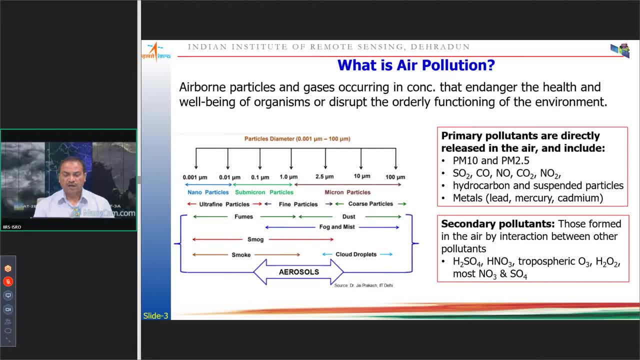 you know, the primary pollutants are in primary nature, that is, that they are directly released from the source in to the air, and the examples are the sulfur dioxide, the carbon monoxide, the oxides of nitrogen, the carbon dioxide and different hydrocarbons and heavy metals. also, there is a very important component. 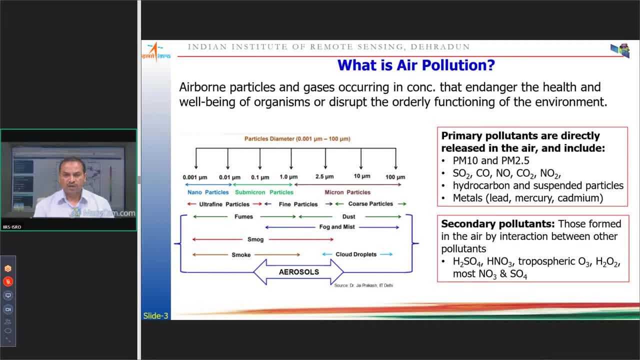 which is known as a particulate pattern. this is a aerosol particle matter which has different sizes. there is fine particulate matter and slightly coarse particulate matter. so PM 2.5 is very fine particulate matter and PM 10 is 10 microns. that is, diameter is 10 micro. all the particles whose diameter is less. 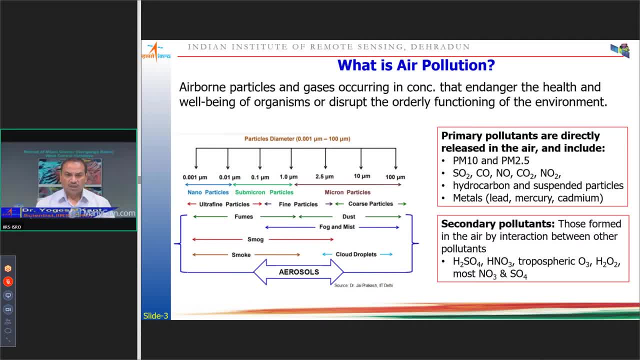 than 10 microns. now if you see the, the different particle diameters as come as respect to the different formations in the atmosphere. now if you see here you the dust, for example, the dust, it, the, the ranges, the size ranges from sub microns to the visible, and the fume. fume ranges from the less than 1 microns. now. 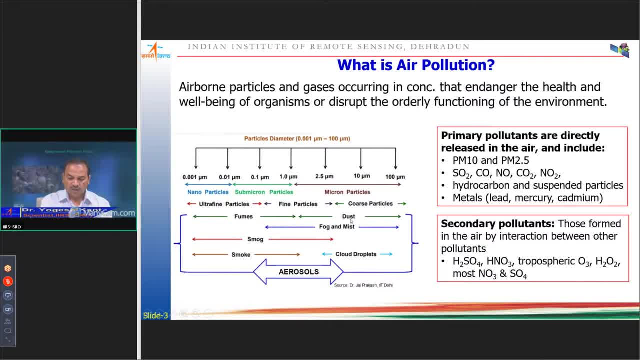 what is dust? as you all know that we can see from dust. these are. this is mechanical disintegration of a parent material and fumes are nothing, but these are produced by condensation of vapors or gases, and then now liquid droplets. when you go about liquid liquid droplets, we have two. 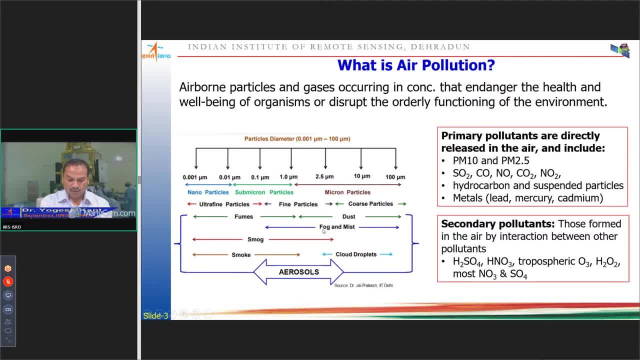 things in this fog and mist. now, if you see the fog, this is the visible nature of the mist. the fog we can see visibly and the mist, mist is somewhat. we can't see this. these are formed by the condensation or the atomization, and this ranges less than 20 or 30 microns. then we have solid. 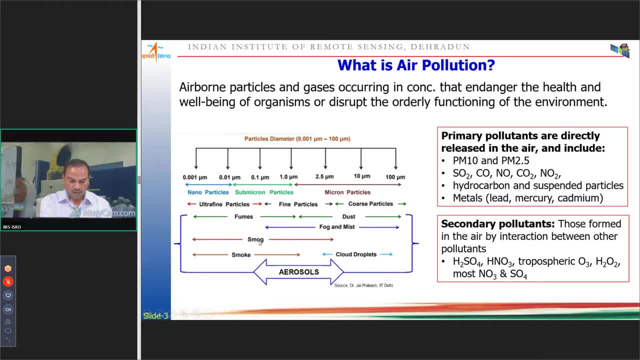 and liquid particulate particle aerosol, and these are the smoke and smog. the smoke, as you very well know, that also can- is visible to our eye and the it is resulting from. the smoke is resulting, as you know, from the incomplete combustion and the ranges is less than one micrometer. similarly, smog- this is: 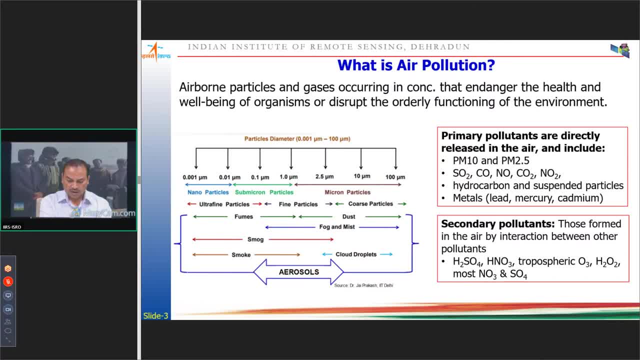 formed due to the photochemical reaction of different chemical pollutants and added with the water vapor, and this ranges less than 2.5 microns and obviously the crouch down cloud droplets. there are larger sizes and it exceeds a around 100 microns. 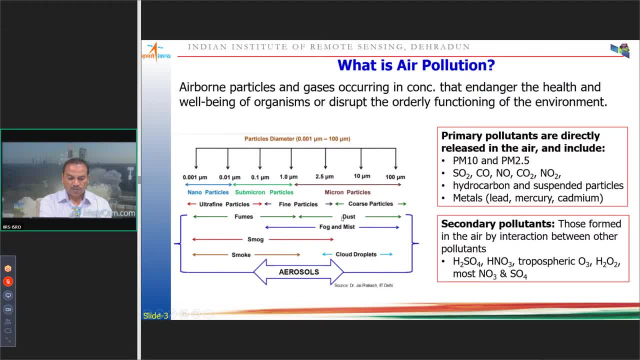 So you very well see that there are different compositions of the aerosols, which are known by different abbreviations, and these particle sizes are less than 0.1 micron, less than 1 micron, less than 2.5 micron and less than 10 micron and less than 100 microns. 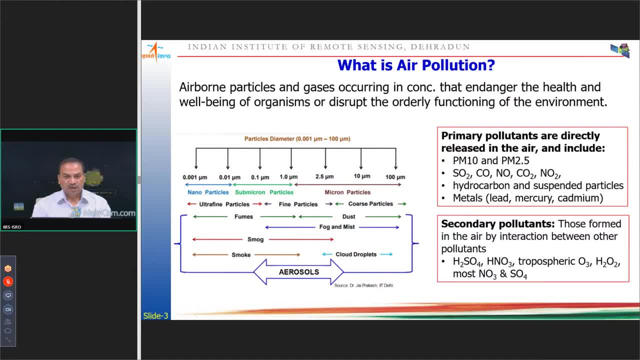 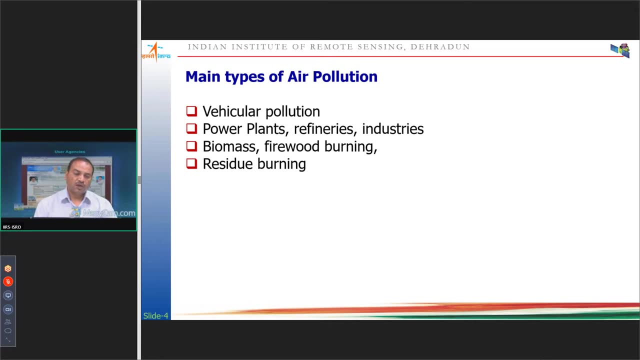 So these have different effects. These are classified. We will see in the next few slides that these are classified according to the sizes. Now coming to the different types of air pollution. Now, what are the different types of air pollution? though, broadly, These are the pollutants which are incomplete combustion from the vehicles, different vehicles. 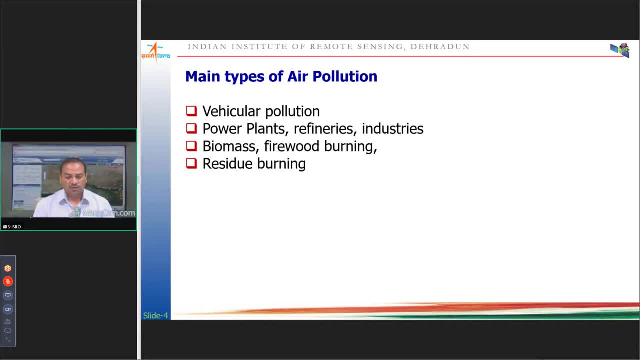 power plants, refineries, industries, The biomass burning, The firewood burning, Then the important is stubble burning, which is known as the residue burning and which is practiced in many parts of the endogenic plane. So many of the pollutants, whether we talk about the ozone, the SO2, the oxides of nitrogen. 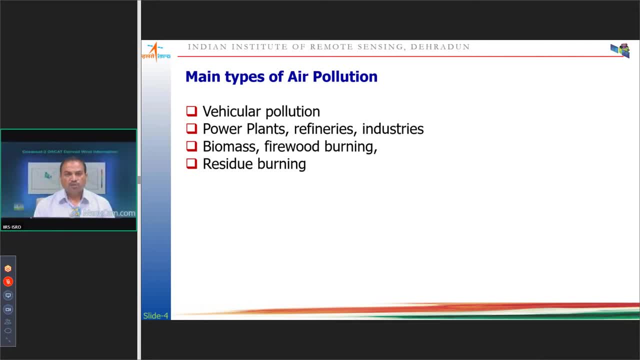 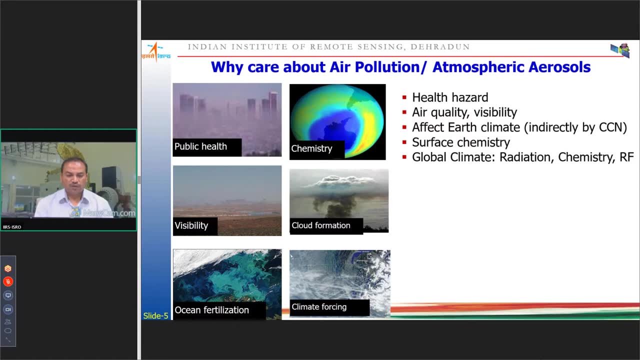 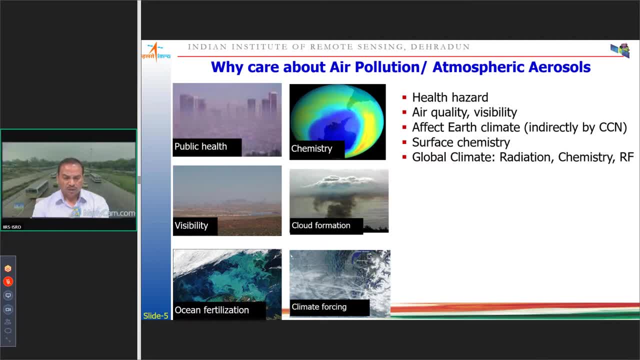 Next slide, Next slide, Next slide. Now the important question that may arise: that this is happening, but why do we care about it? So why do we learn about it? All the about the air pollution and the aerosols and all that. 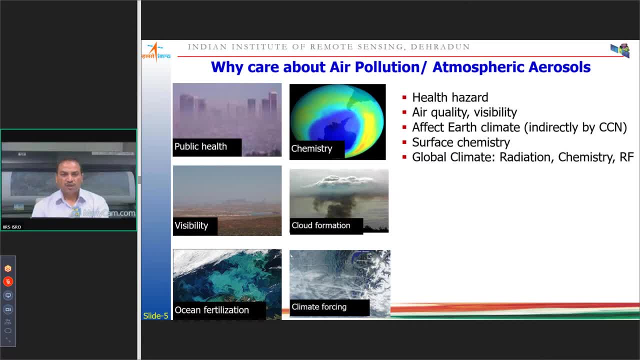 So I have classified broadly into these categories. First is, obviously it is harmful for the wellbeing, like, for example, human human health or the vegetation. So the public health. So the public health, Why? Why the? the particulates? the particulate matter whether it is a form of a nitrate, sulfates. 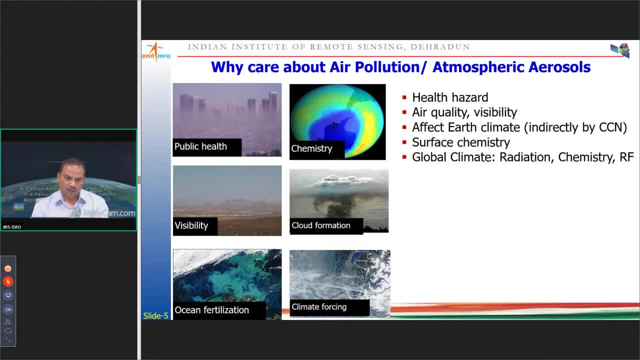 organic compounds, metals, soil, dust, so these are affecting directly to the human health. so we inhale it and it goes in our respiratory system and then it becomes. it is toxic in nature and it is leading to many chronic diseases. uh, broadly, two point: pm 2.5 is known as the respirable. 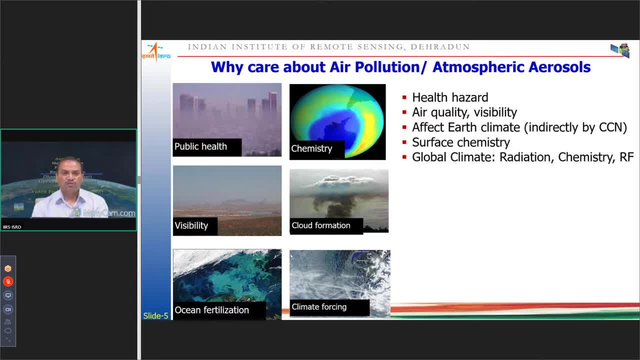 particles, because it is very fine particles and naturally our nostrils cannot stop this. and though they penetrate through our respiratory system to the lungs and then- and they have a very toxic nature- and react in our body for and they cause many diseases. pm10 is known as thoracic particles, and these are also harmful for the human health and the 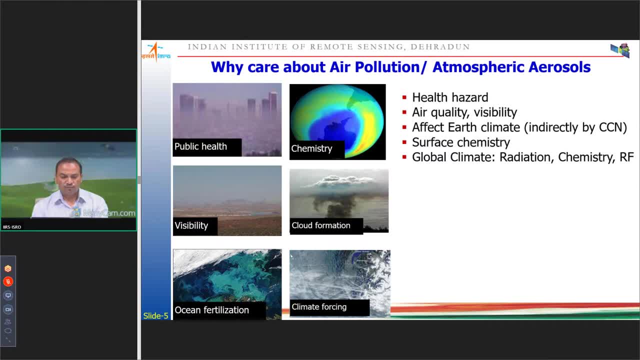 another. the problem of the aerosol or care, the, is the surface chemistry, the change of the surface chemistry and the atmospheric chemistry also. so these affect the and the, the secondary form of the aerosol, they. they are chemically reactive and then they oxides, make the aerosol and then they oxidize, and then they oxidize, and then they oxidize and then they. 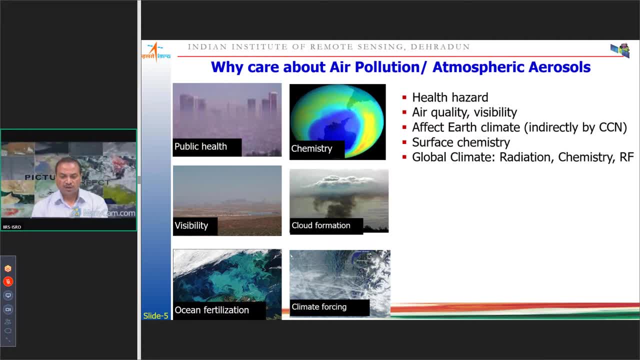 many uh oxidations and then their formation of the secondary type of aerosol which affect of the earth radiation budget. also, uh it is affecting the visibility and like fog, mist and visibility. so the day-to-day life, the economically uh the it is affecting and creating a loss. 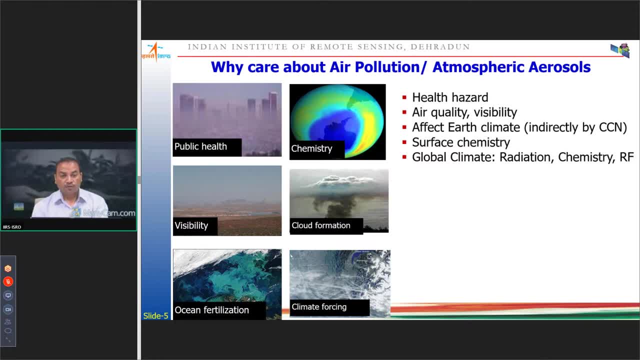 for the economic growth of, for few days or few months, of a country or a region. uh, also the it is affecting the oceans because the they dissolve in the ocean, these different components of the aerosols they dissolve in the ocean. and affecting the change in the ph. 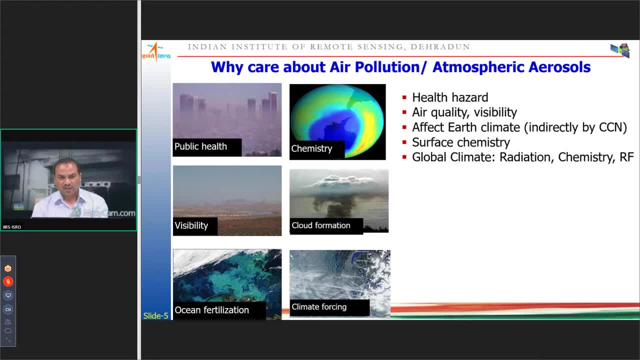 value, so the it becomes more acidic and when many aquatic species they react because most of the aquatic species they are the carbonate. when, when the carbonate is released, they are, the carbonate reacts with the acidic, so there is a disintegration and there is a problem for the aquatic species. 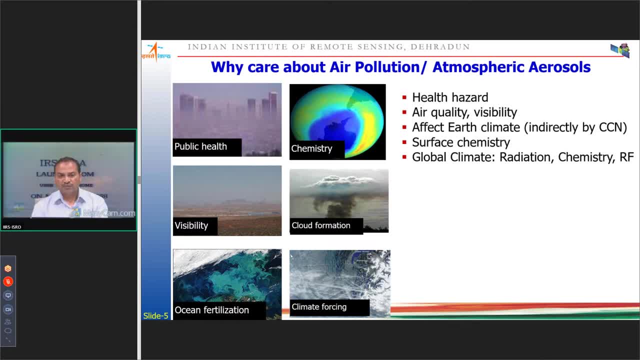 so the ocean, the. it has a adverse effect on the ocean fertilization and change in the ph value. also, more aerosols means more condensation nuclei and more formation of the cloud and in fact indirectly there will be more scattering of the solar radiation. so less amount of amount of. 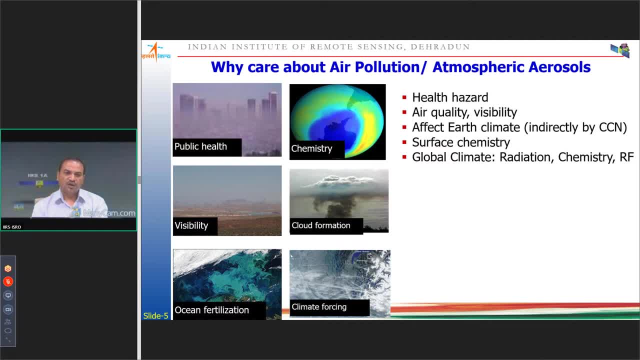 radiation reaches on the ground and thereby it is having a net cooling, or the change in the relative forcing, also the in totality, the climate forcing. when you take about the, what is the amount of the total relative flux? so in totality, the climate change and climate forcing. so it also 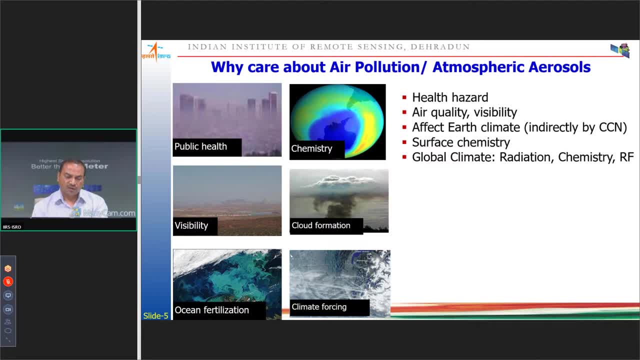 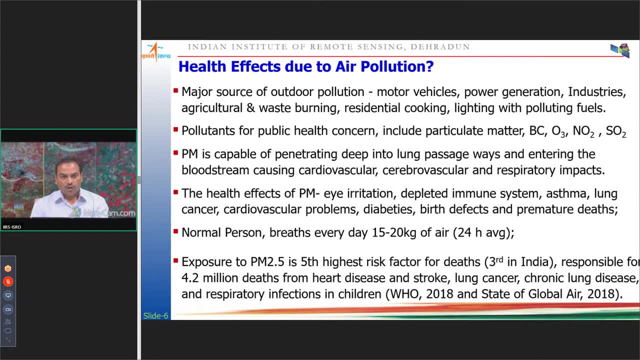 plays an important role in adverse, adverse effect of the climate forcing. now this focuses on what are the different health effects due to the air pollution. so we know that now most of the people, now, in fact, the children, also know that now the air pollution is creating the health hazards, the major: the outdoor pollution, indoor pollution, and both are 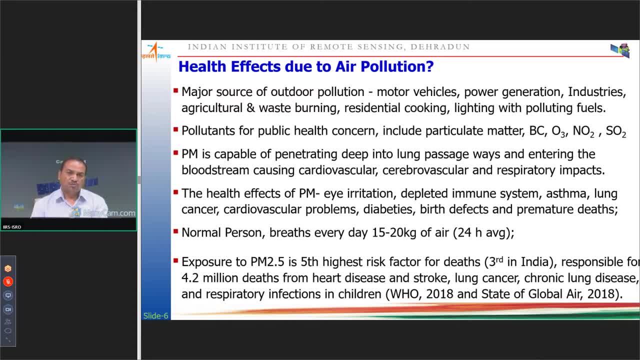 dangerous and these are mostly, as i said, mostly produced from the motor vehicles, power generation industries, agriculture, waste, residential cooking and the different kinds of fuels, what we use and these, particularly the black carbon, the particulate matter, ozone and o2 and so 2 and these particulate matter, particularly they, as i said, they penetrate deep in the lungs. 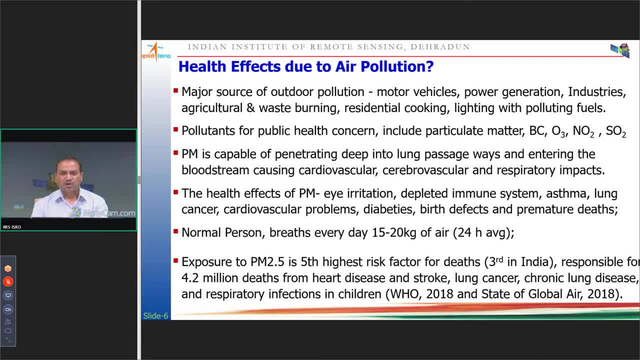 and in the they go in the bloodstream and a lot of cardiovascular problems and respiratory problems. respiratory, respiratory problems are affected by it and particularly from infants, children less than five years, to young age, to the old old age. so everybody is affected by it. the common symptoms: what is the? having the? 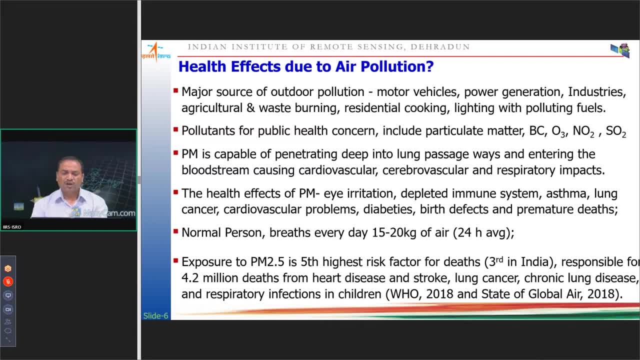 irritation of the eyes. eyes irritation when we are more exposed to the pollution, whether it is indoor or outdoor, both, and it also the more exposure also depletes our immune system. the common is the asthma, the, the lung problems and lead to the cancer. and also recent studies show that most of 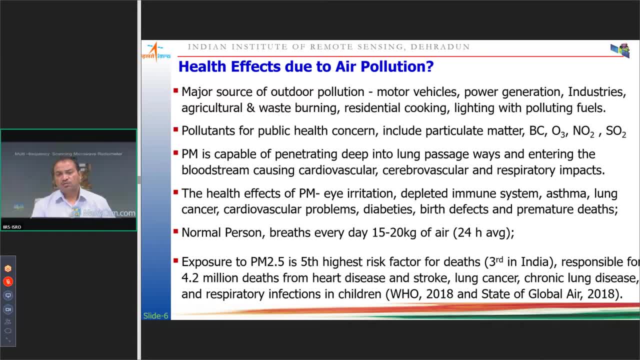 the diabetic patients are those which are who are exposed to the most of the hazardous pollution areas. so this is the diabetic diabetes also being the concerned by the effect of the pollution and the, the birth defects, the pregnant ladies- this also affects it- and also the premature deaths, less than two years infants or the five years children just. 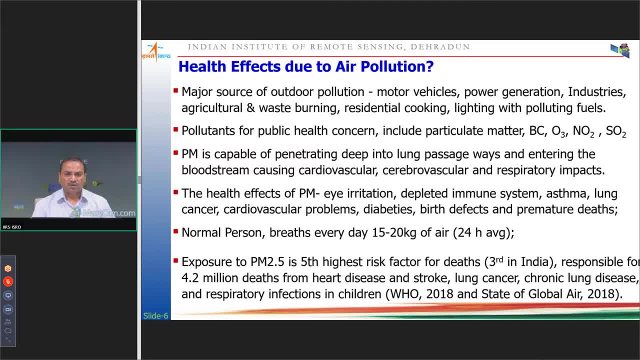 an in for the information. I just put that a normal person, we breathe in a particular day 15 to 20 kgs of air. now if this air, if five percent, ten percent of it is polluted, so how much effect it happened it has on our- you know- whole of the body and different organs, just for the 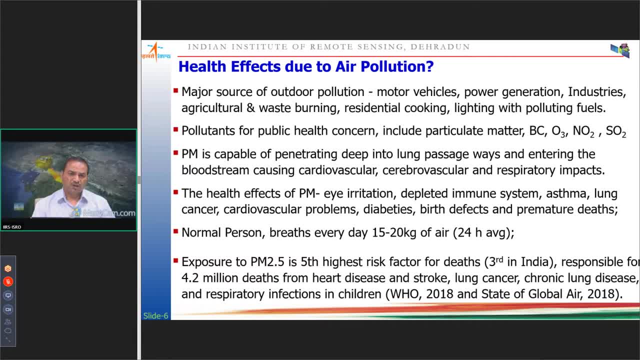 statistics: the exposure to PM 2.5, which is very dangerous. that is the fifth killer in the world, and the fire and feist high, highest risk factor and which is third in number, that is the the third highest deaths are being recorded by PM 2.5- is responsible worldwide for 2.4 point 2 million deaths from different. 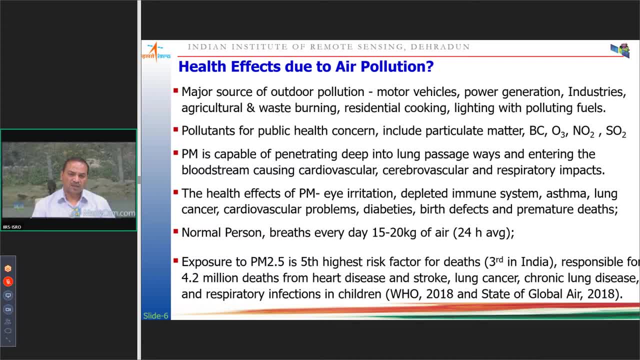 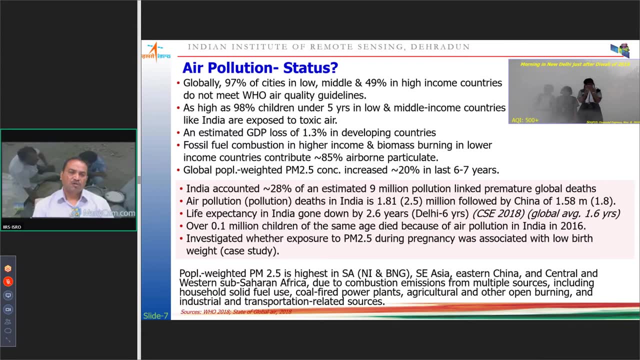 kind of heart disease, different kind of heart disease, diseases like heart disease, stroke, lung cancer, chromatic and other things. so it has becoming in concern and that's why worldwide people and organizations and country level, the policymakers are incorporating how to tackle the air pollutions. this is a 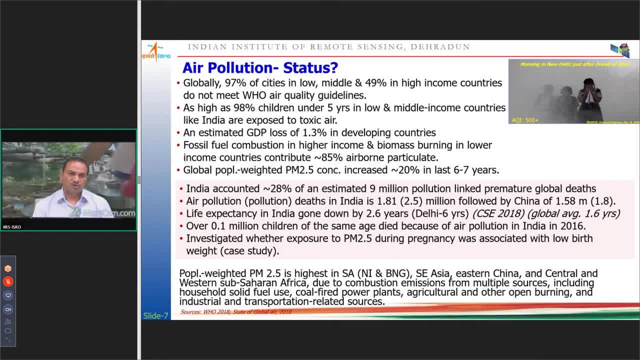 glimpse of the statistics of the air pollution are particularly focusing on in India, if you see here as 98 percent children below five years in low and middle income countries are affected, like like India. so around 98 percent of children are exposed to the toxic air. again, if you talk about indoor, indoor also is polluted, outdoor is also. 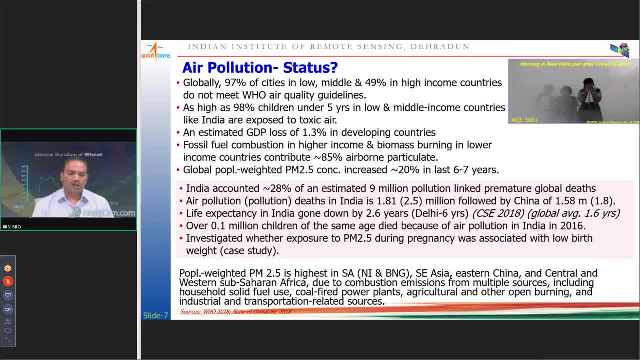 polluted both and not only affects the human health, but also it affects the health of a country, that is, the economic health- around 1.3 percent of GDP in developing countries. it's there is a loss of for it and the most of the fuel fuel, the fossil fuel consumption and the biomass burning their attributes around. 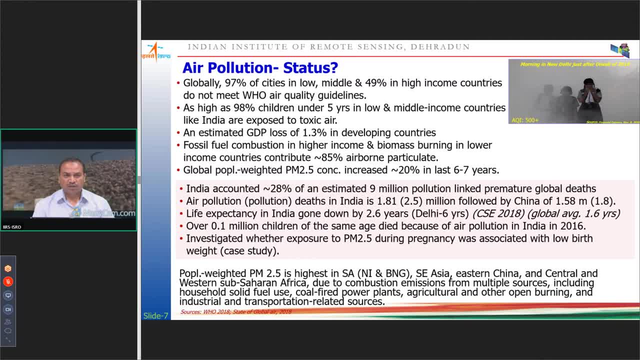 85 percent of the airborne particulates which is emitted in the air and if you see the global population weighted PM 2.5 concentration average, so last six to seven years it has increased by twenty percent. so more, more, more of the pollutants, more of the vehicles on the road, more industries. 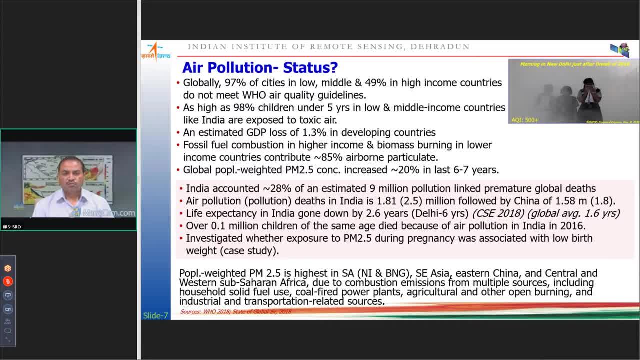 more economic growth and more of the pollutants are there in the atmosphere. India accounts twenty eight percent of the estimated nine million population deaths, premature deaths and India, and in India the deaths are highest in the world. air pollution is 1.8 million, which is for then followed by the China one. 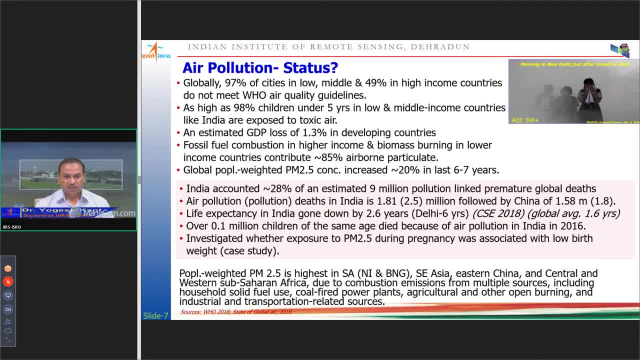 point five million and due to this, the life expectancy has decreased by 2.6 years and in Delhi particularly, it has decreased by six years now, you see, and global average is around 1.6 years. so that is the concern and that is the alarming rate, which is the air pollution is affecting our day-to-day life and the 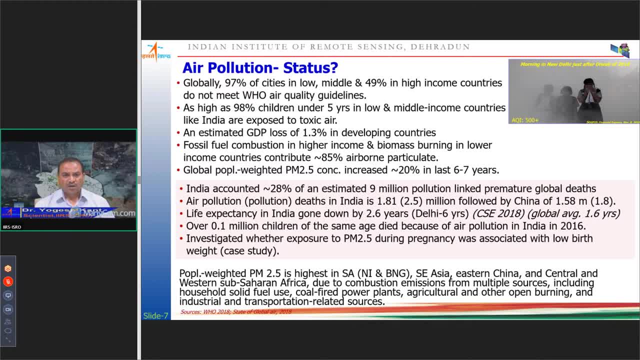 health and our children. as I said, there are many case studies over India where the effect of the PM 2.5 on pregnant ladies. so one such study was taken in southern India and which shows that, due to the the, the exposure to the PM 2.5. 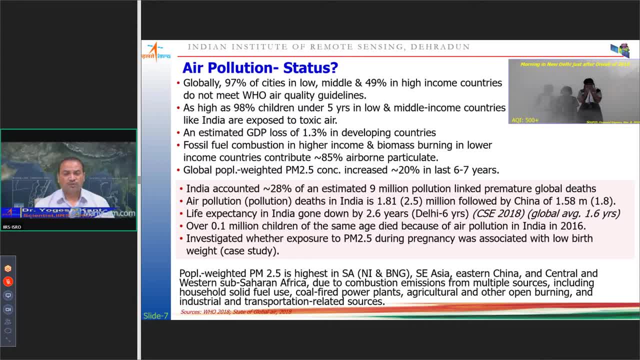 has the low birth weight of the infants born and, as as a region is concerned, the weight a population weighted PM 2.5 is highest in this South Asia, particularly the northern India and Bangladesh, and also in the Southeast Asia, Eastern China and central and sub-sahara. 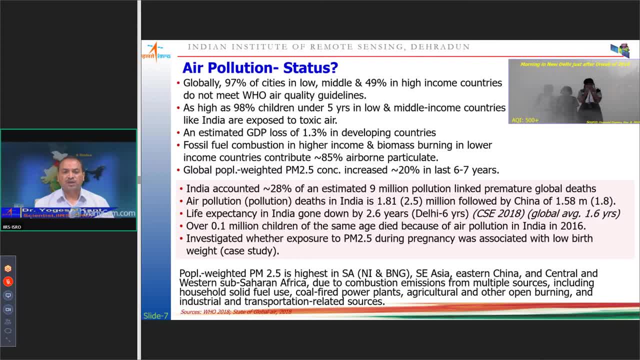 Africa. now this central and sub-sahara is a dust. it comes to dust because there are Saharan dust and many months it is affected and it travels to thousands of yaşa and thirty to fifty than the average age of the population in Asia. kilometers to Southeast Asia, including India, of course, and, as I said, the 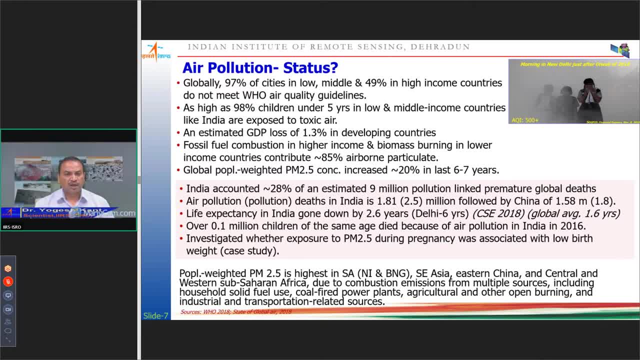 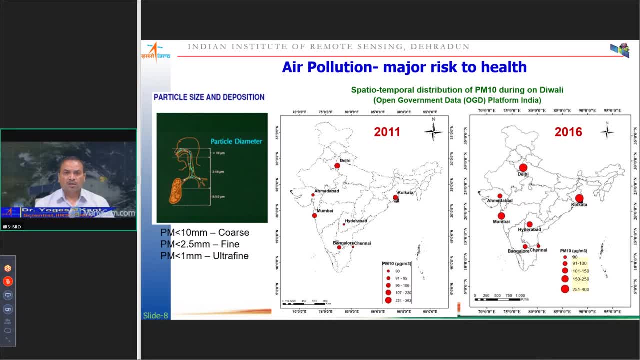 sources are vehicles, power plants, power plants, agriculture, residue burning and so on. now, if you take about India, I put around seven, six to seven major cities. in the last six to seven years it has doubled. if you see the statistics from the. these are central pollution control board and the 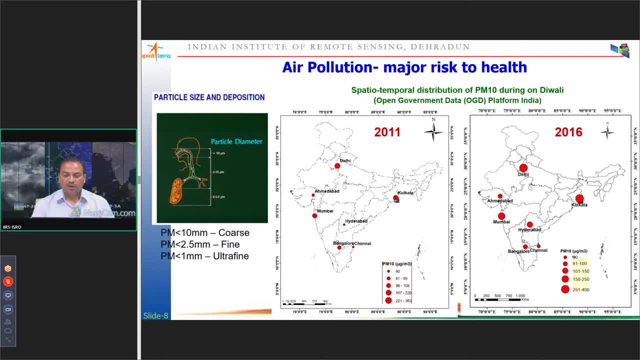 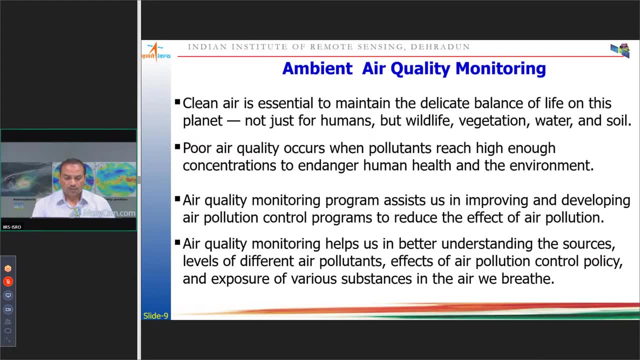 the PM 10. on PM 2.5, they have increased to almost 100% now the now ambient air quality monitor. so so all these put together, now what we should do. what we should do is: first example: we should to know the concern to, to know the alarming rate. first of all, we should try to understand it. 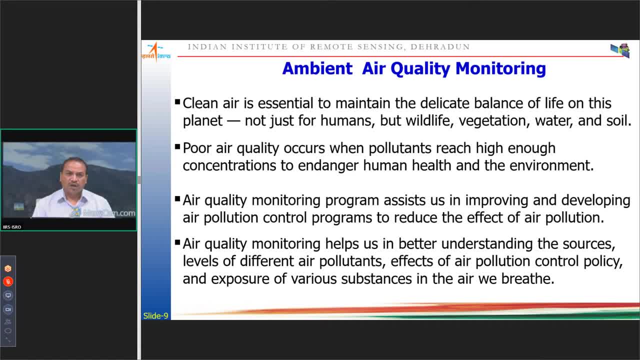 understand the process, what they understand, the culprit and how do we tackle it. and then, as a policy, we have to understand or keep on, keep on monitoring the quality of the air. now, as I said, the pollution, a air which is above a threshold, the pollutants, the concentration is above a threshold. we 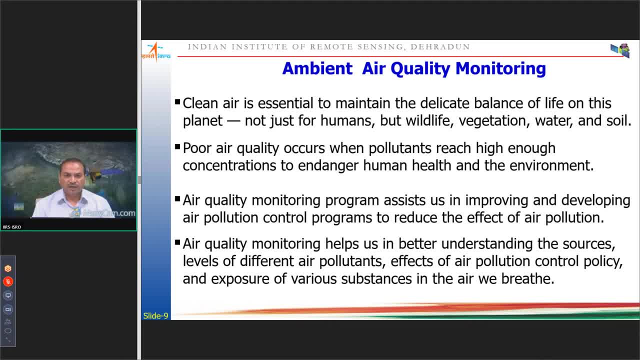 say, as it is a pollution, but below the threshold it will be clean air. so all over the world, different countries are adopted national standards of different pollutants and then there is an continuous monitoring of different cities and we say that ambient air quality monitoring, now it is essential. 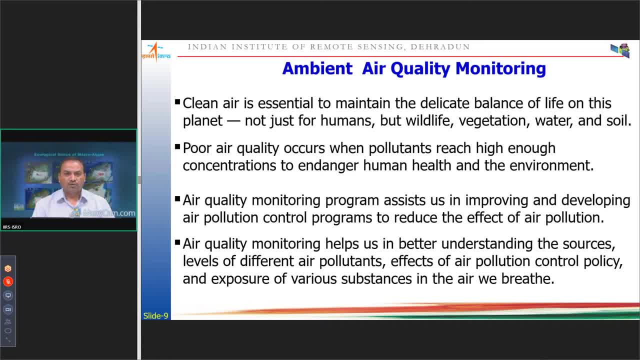 as I said, to see the balance of the between our environment and where we live in. we have humans, wildlife, vegetation, etc. etc. and the, the air quality monitoring program, which assist us in improving and developing the air pollution control programs to reduce the air pollution. now also that the the purpose of the air monitoring is not 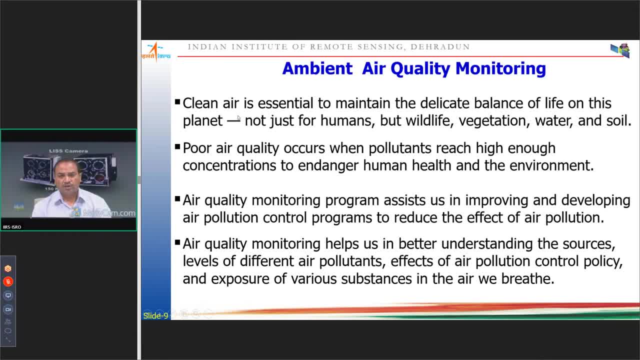 only to measure it or to collect the data, but also to provide the necessary information to our researchers, the scientists, the policymakers, then to planners to make decisions and to you know, to manage how to improve our the, the the quality of the air also, these air pollutants also. 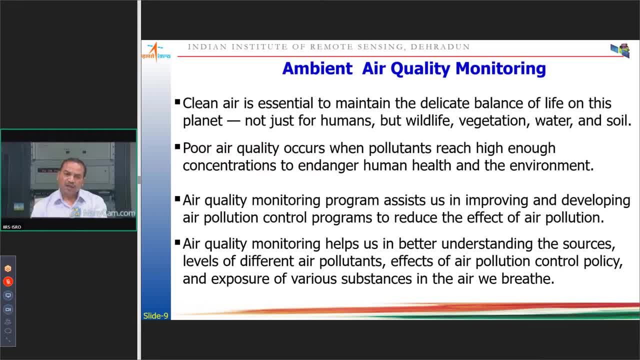 are acting as indicators and this information is also made widely public because people also should know what is the, what is the status of the quality and what steps has to be taken on all that. so the air quality monitoring is not for the researcher but also to to make public and to make an awareness program to aware people. 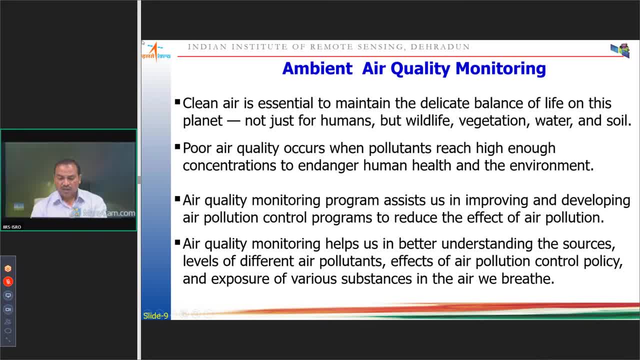 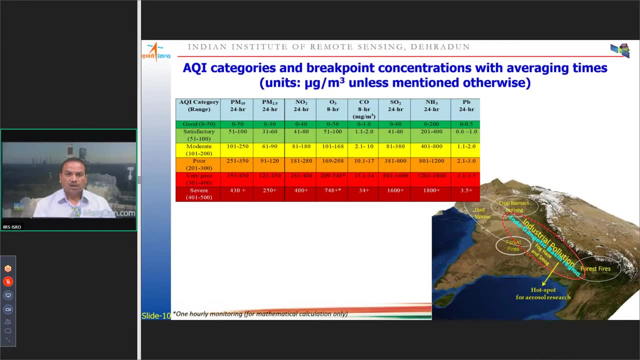 and they aware the citizens at different times and so that at each individual level, at citizen level, they can also take their decisions. I think in the last class also, you must have been aware about the different categories which air, air air quality is concerned. so how do you know that our air quality is clear or polluted? so we see the 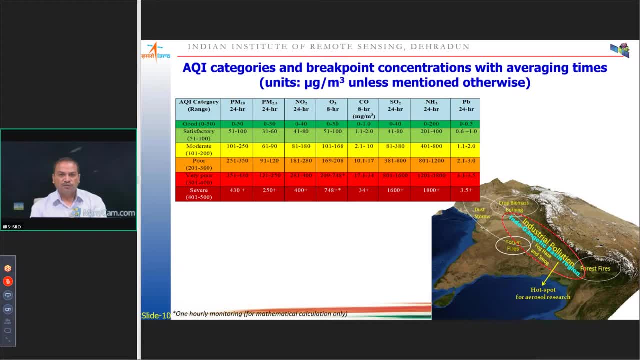 central air quality is clear or polluted. so we see the central air quality is clear or polluted. so we see the central pollution board, which is a centralized agency for data collecting and monitoring. they have come out with an index which is known as the air quality index. so if it has a different categories, 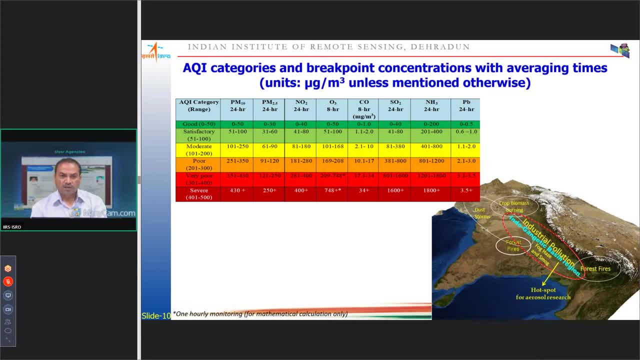 and there are different eight major pollutants which they measure continuously. measure different stations all over India continuously over 24 hours. it is pm 10, pm 2.5 and o2 stations all over India continuously over 24 hours. it is pm 10, pm 2.5 and o2. 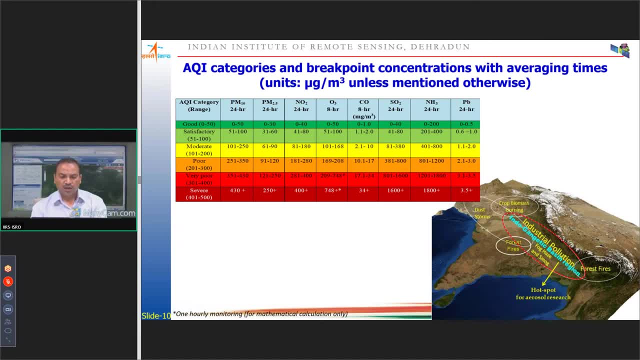 ozone, carbon monoxide, sulfur dioxide am on NH 3 and your lead, and out of these ozone, carbon monoxide, sulfur dioxide am on NH 3 and your lead, and out of these, there are four major pollutants which are measured by all the stations: pm 10. 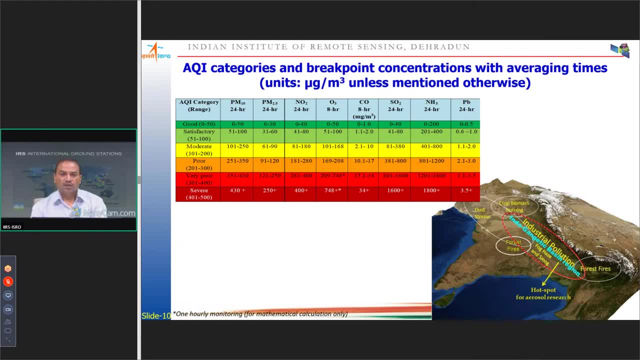 there are four major pollutants which are measured by all the stations: pm 10, pm 2.5, so 2, ozone, these are all measured continuously, or old stations and some stations. they measure all eight parameters. now, different categories: the air quality index from 0 to 50. air quality index from 0 to 50. 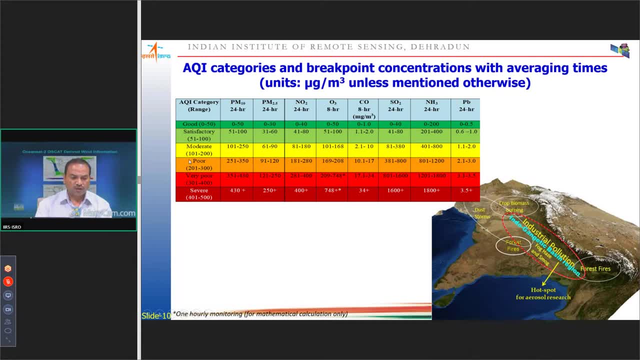 is good, 51 to 100 is satisfactory, and so on. now it becomes. when it becomes more than 200 becomes, or 200 to 300, it becomes poor, and and when it becomes 300 to 400 it becomes very poor. so it is an alarm. so the citizens, or the public, and 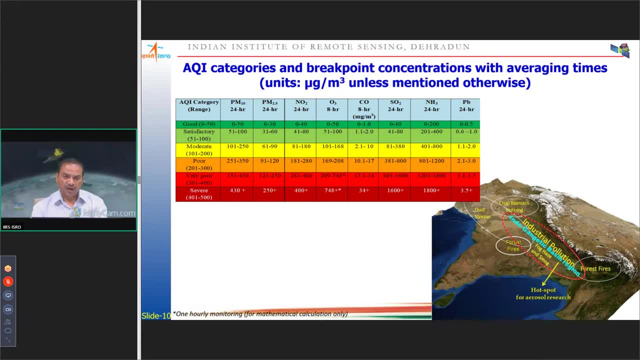 the local administration. they give alert and it is like orange to red, so color also is changes and it is an alarming. and then people has to decide whether to stay at home to reduce their traffic and so on. and when it crosses the 400 mark, the AQI coins 400 marks so it becomes severe. so it means the, the local, 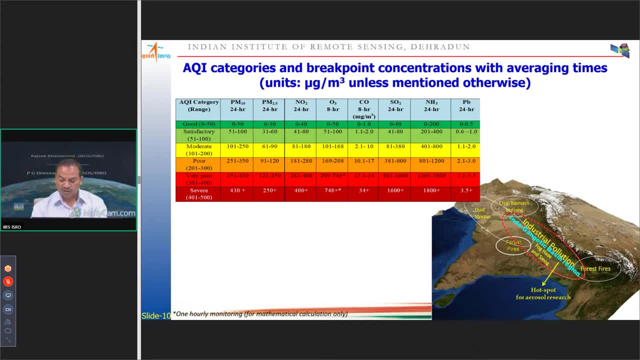 administration can take decisions. so it is a very severe status and it means that it is hazardous to be exposed in the outdoor pollution and and needs an immediate intervention by the local authorities and by the public itself and they have to take decisions. the another left the figure which shows that what are the different kinds of the sources. so the 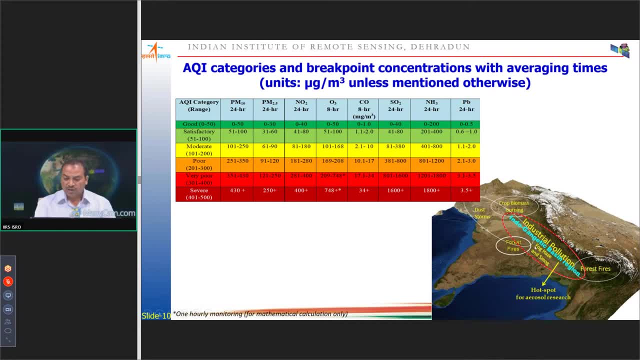 this is the indo-gangetic plane, the, the Western Indo-gangetic plane, the central Indo-gangetic plane, the eastern Indo-gangetic plane, the Western Indo-gangetic plane is influenced by one or one is dust storms, which is coming from the. 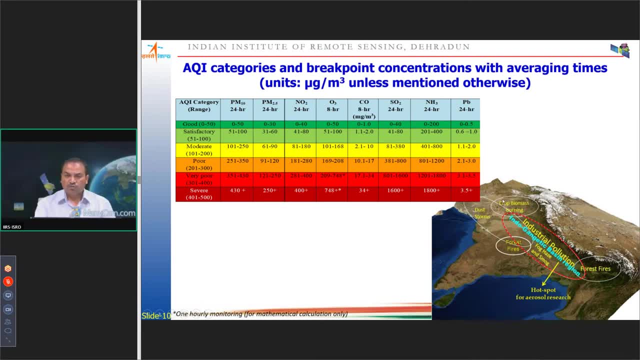 North Africa from thousands of kilometers and it travels to upper layers and camouflages the larger areas of the Indo-gangetic plane in northern India. the another source is the, the crop burning, that is, the residue burning. it happens in the Punjab, Haryana and Western Uttar Pradesh and then mostly in the 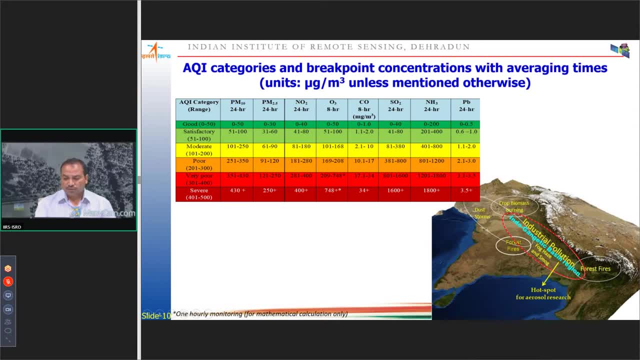 post-monsoon season and also in the pre-monsoon season. then there are different sources: from the forest fires, which is from the northern India and burning of the forest fires creating the NOx, so to and particulate matter, and there are many industries because it is highly population, populist, area, region in. 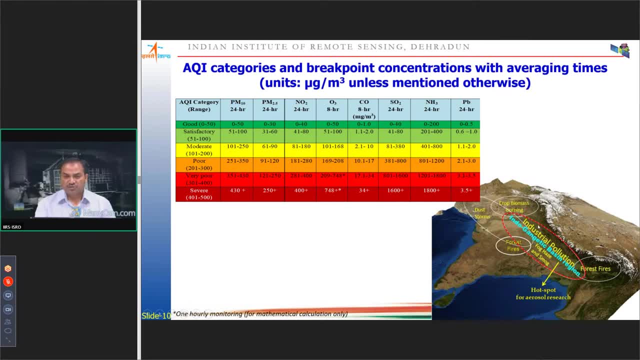 the Indo-gangetic region. so we have a lot of industries, power plants, so the pollutant from there and also the meteorology of this area is, as such, the there is the occurrences of the fog and the small and the, particularly in the winter season, so this region is particularly very hot spot. 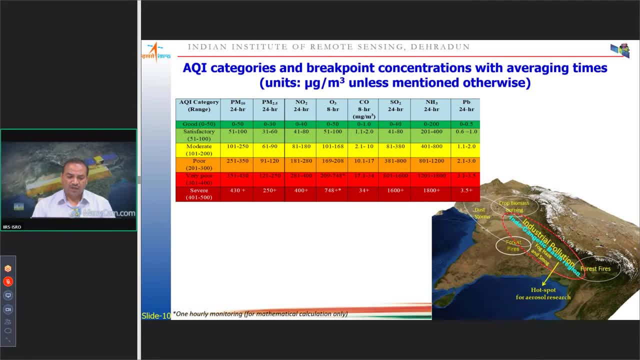 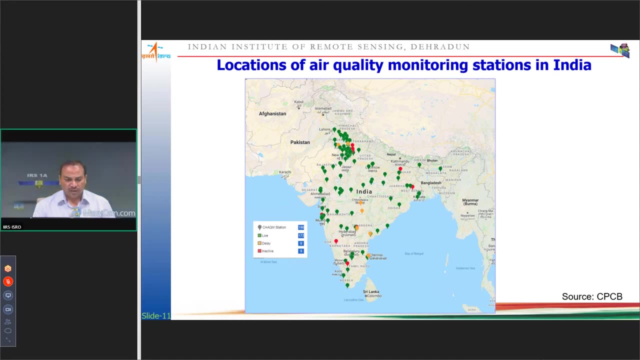 and most of the cities in this region are affected by the deterioration in the air quality, and the air quality is a must to monitor all the areas. this I've taken from the Central Pollution Control Board website so you see different kinds of stations, locations, as they have the geographic latitude, longitude, name of 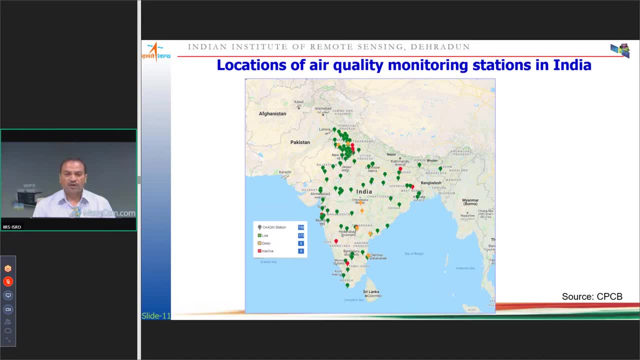 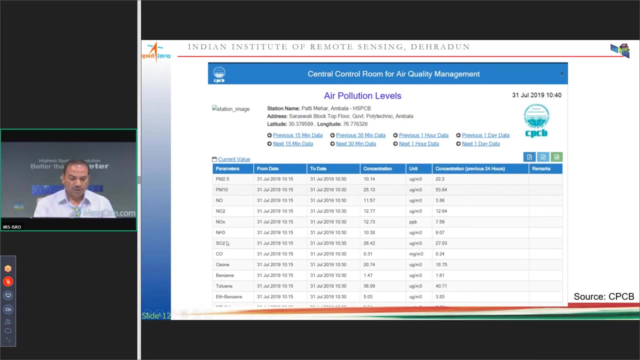 the stations, what they measure, what are the different data they provide, how long the data has been existing in all these stations. so all these is easily and freely available over the net, like I told you. PM 2.5, PM 10- so so many parameters they measure, and also the benzene, toluene and all different kinds. 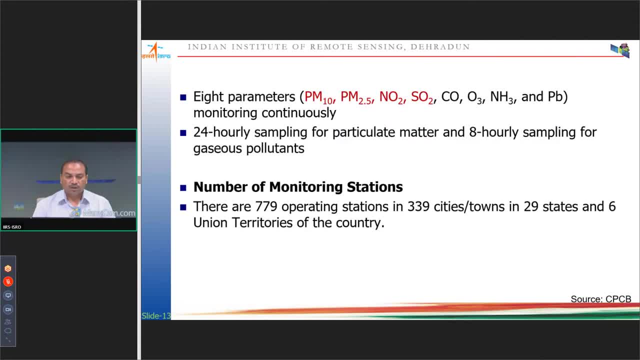 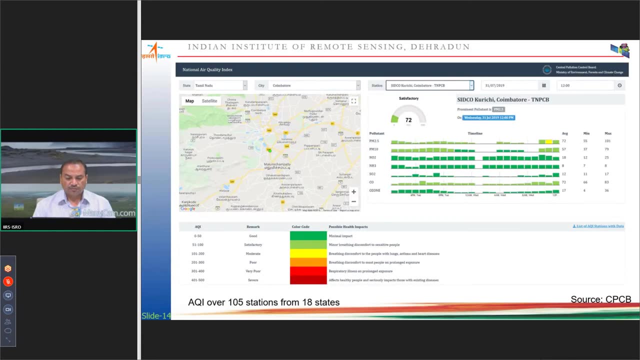 of hydrocarbons of the minute they measure. so they are operating over India around 780 operating stations in 339 cities and 29 states and 6 union territories of the country. and this is the live example of one of these stations in Tamil Nadu, Coimbatore. so they gives the hourly values and you can. 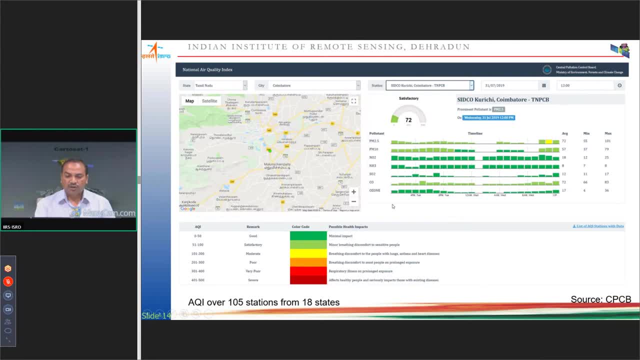 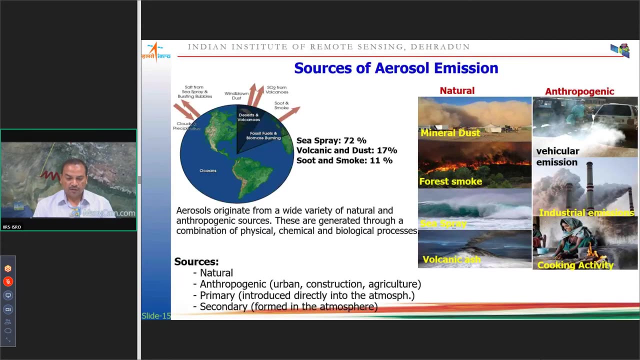 monitor the life, what is the current value of the stations and what is the different parameters or these each stations and this color exists. this coloring code is as per the air quality index. so green is good and moderate, like green. so now the sources. as I said, the sources are won by as a three-fourth of the 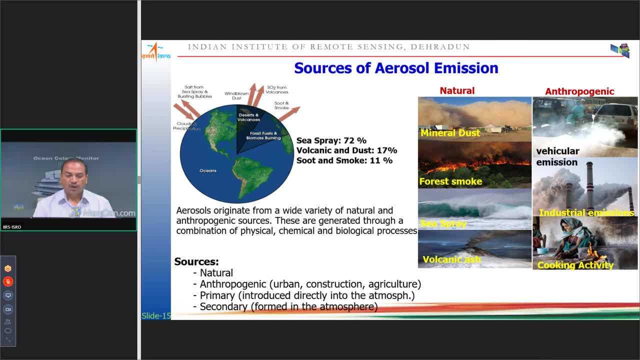 earth is covered by ocean. so most of I I said these are natural and anthropogenic. so most of the aerosol emissions are natural. around 85 percent of emissions are natural and around 15 percent is from the human or activities or anthropogenic. but it is increasing. 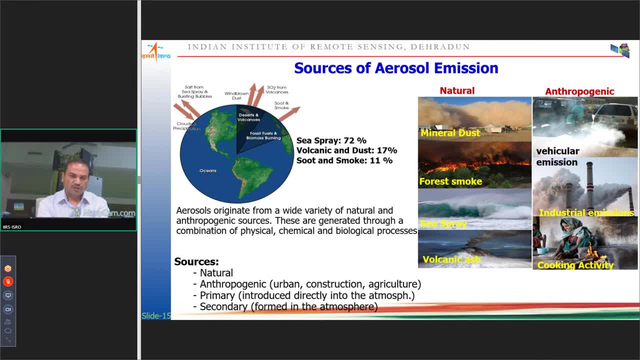 day by day and year by year. and the anthropogenic component is increasing. the sea salt is around 72 percent, aerosol- the volcanic is just- is around 17 percent and the anthropogenic suit- a smoke- is around 11 to 16 person. as I said, the natural is large and the anthropogenic is small, but the, the, 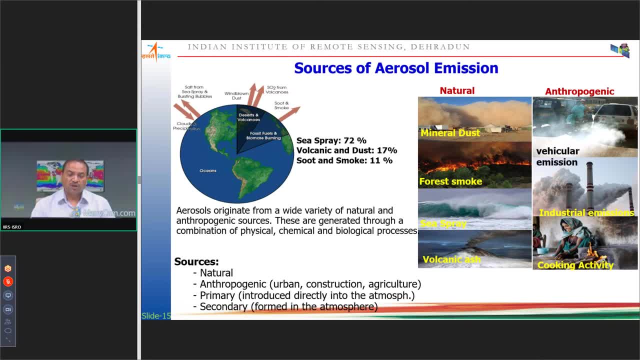 effect of the anthropogenic aerosol is huge because most of the fine aerosol which is emitted is only from the anthropogenic activities, whether it is pm 10- oh sorry, pm 2.5 and pm 10 is mostly by anthropogenic 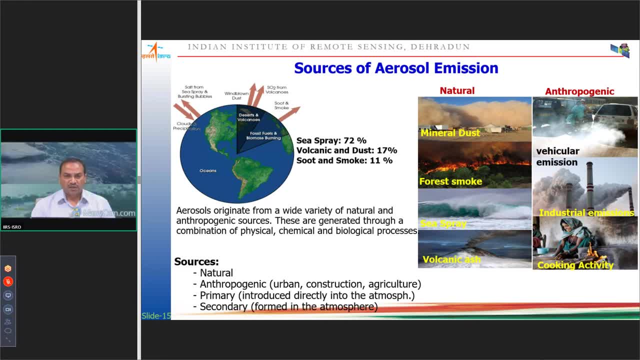 and well, 아까 kita dosa, hatip nur terima. And the coarser, that is, larger particles, are from the natural aerosols. So most of the effects which is notified either on the human health, the fertilization, ocean fertilization, the change in the pH value, the climate forcing, is mostly affected by the fine particulates, which is from the anthropogenic activities. 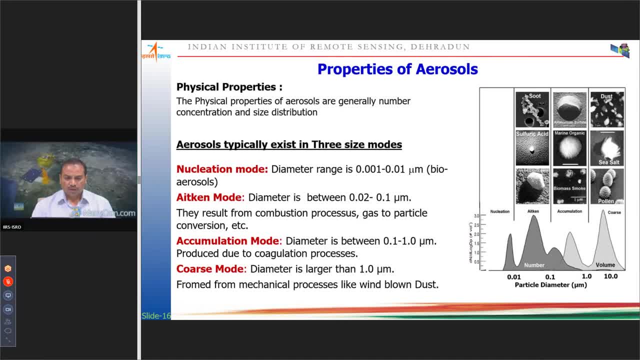 Now, as I said, the aerosols are classified according to the sizes They have. the nucleation mode, that is, diameter, is 0.001 to 0.1 microns. The Atkin mode, that is 0.02 to 0.1.. 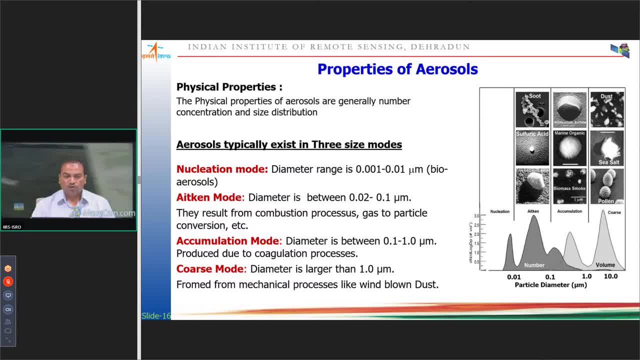 The accumulation mode, that is, 0.1 to 1 microns, And the coarse mode, the larger is all particles greater than 1 microns. Now, this is the accumulation mode. This is the accumulation mode. This is the picture taken by the electron microscope. 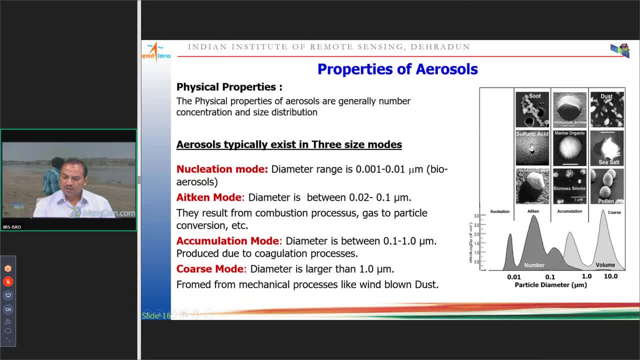 You see the soot, the dust, the marine, the sulfuric acid or the sulfate aerosol, sea salt aerosol. Certain aerosols are spherical in size and certain aerosols are not in spherical size, So the physics of it will change. 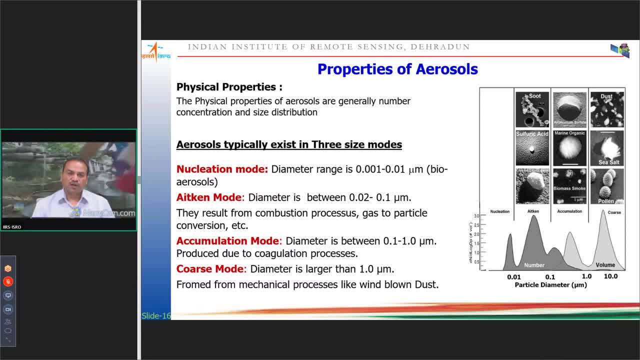 Because most of the physics, it is assumed that most of the particles are spherical in nature, But in reality some of the The aerosol particles are not spherical in nature. Hence we need to understand the shape, the geometric shape of it and try to understand the interactions of the electromagnetic radiation on it. 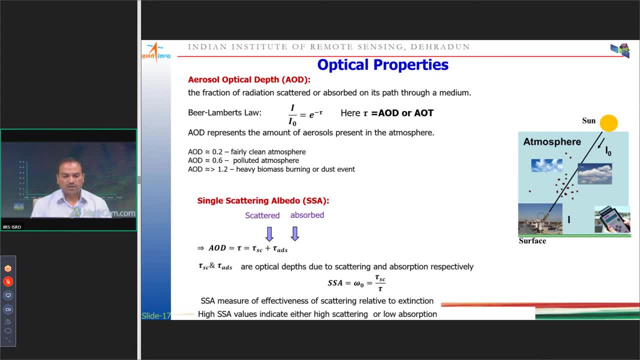 In terms of the optical properties, that is, the interaction with the electromagnetic wavelength. we know that there are the scattering and absorption, Now the scattering. In the scattering there is a change of the wavelength and the absorption also the change in the direction. 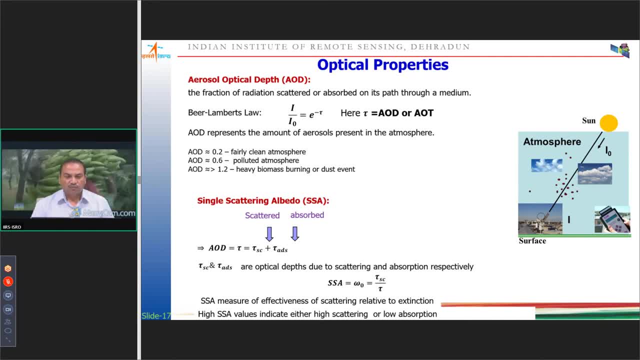 And now what happens is, when there is interaction, there is a component of these two which is known as extension. Now, the degree of extension depends on the medium which it is interacting, And it is governed by the equation from the Lambert-Beard law and which determines the extension depth. 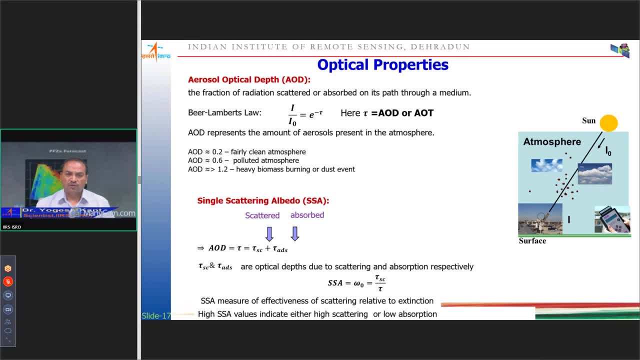 or what is the degree of the extension or the degree of the scattering or absorption happening on that particle And which is denoted by aerosol optical depth, by term, or we say as AOD, aerosol optical depth, or aerosol optical thickness, or AOT. 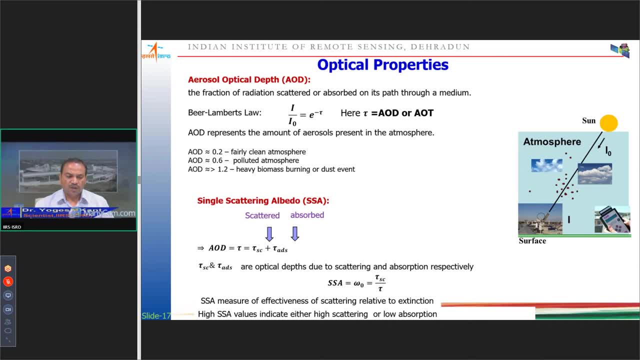 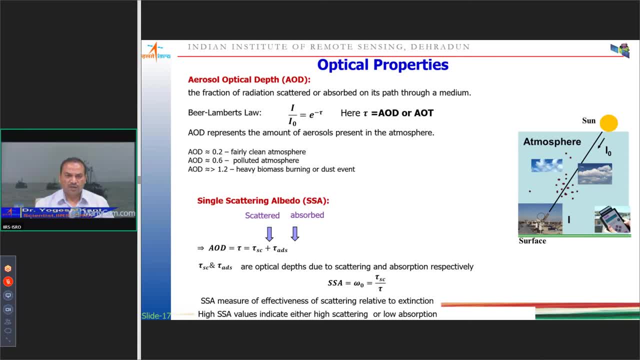 So we say that it is more or less a cleaner atmosphere, that is, pollutants are less than the certain standards. AOD is around 0.6,, so it is a, you know, slightly polluted atmosphere And if it is like, for example, more than 1 or more 1.2,. so there are. 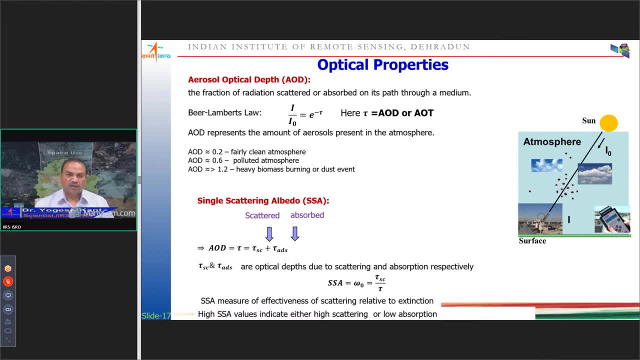 It is heavily polluted. So these are some of the indicators with which. So these are some of the indicators with which we can say that the air around us is the level of pollution, how much it is. The another optical property is the single scattering albedo. 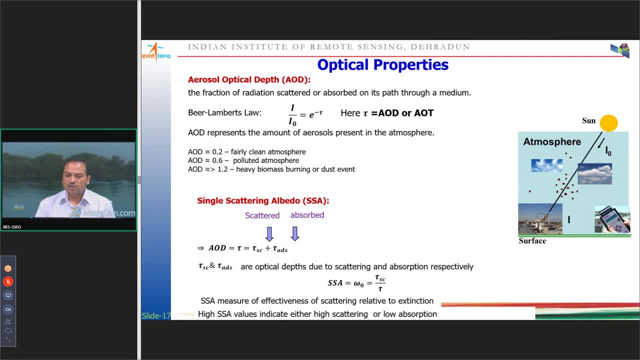 These are: This shows the depth of the. What is the depth of the scattering or absorption of In a particle? So it measures the effectiveness of the scattering relative to the extension. So if the SSA is high, So the 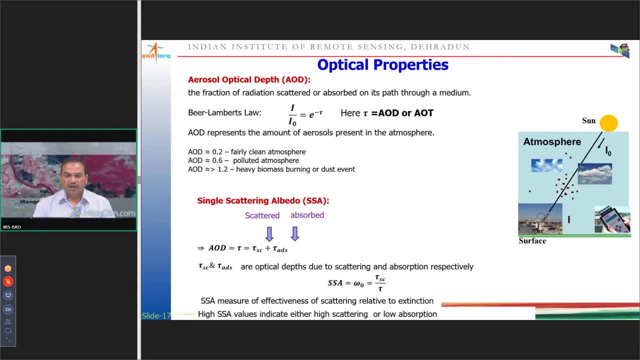 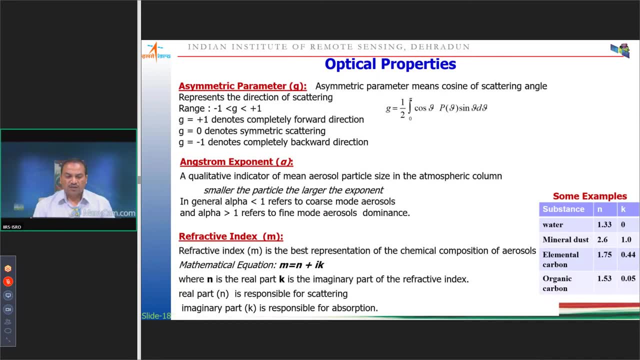 It means the scattering is more, or that particle nature is more of this scattering. Another property is the asymmetric parameter, which gives the scattering angle, or whether scattering happens in the forward direction or in the backward direction. The Angstrom exponent. The Angstrom exponent. 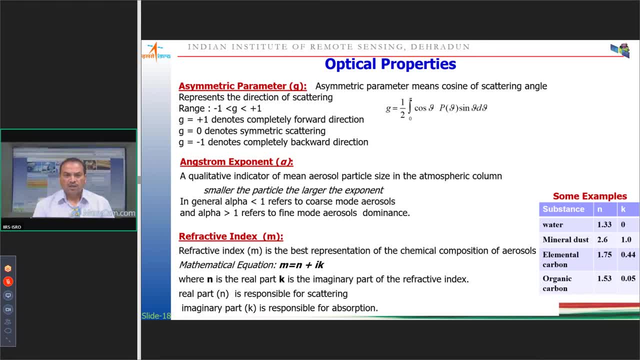 The, The, The. The determines the mean aerosol particle size. so what is the aerosol particle size? whether it is a small particle size, accumulation mode, fine mode or a coarse mode. so roughly, if the, the angstrom exponent value, is less than 1, it means 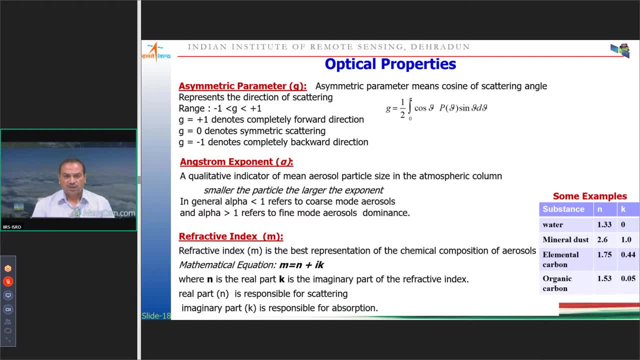 it is the particular, the particulate, which is the particle which is interacting with the algorithm. tradition is larger or coarse particle, or if the value is greater than 1, it means the particular smaller in size or fine particles. also, we can also estimate the refract from the refractive index also. 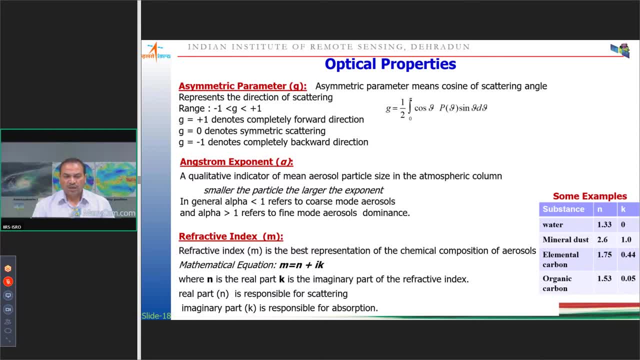 we can estimate whether the nature of the particle is more scattering or more of a absorption in nature. so the the real part an imagery part. so we define from the real part the scattering nature of the particle and from the military part, where we understand the luminosity value which is an image når. 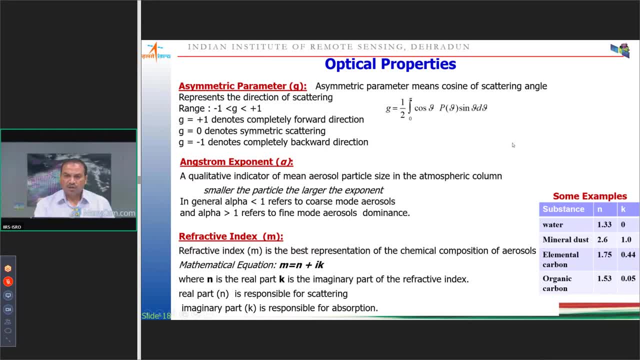 the absorption nature of it. for example, if you see the water, the, the water, the refractive index is 1.3 and it means the the real part is 1.3 and imagery part is 0, so more towards the scattering nature. but if you see the organic carbon or for 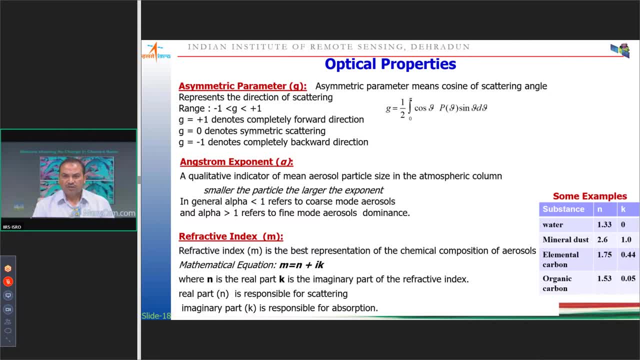 example the elemental carbon. so 1.75 and 0.4. it means a substantial portion of absorption is also there. so it has both the absorption and scattering and both. so it's a very complex aerosol particle. nature is very complex to understand it. it's a mixture of many components so you can't say as if it is more towards a 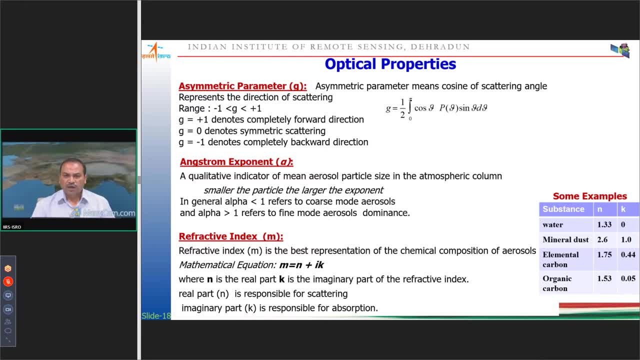 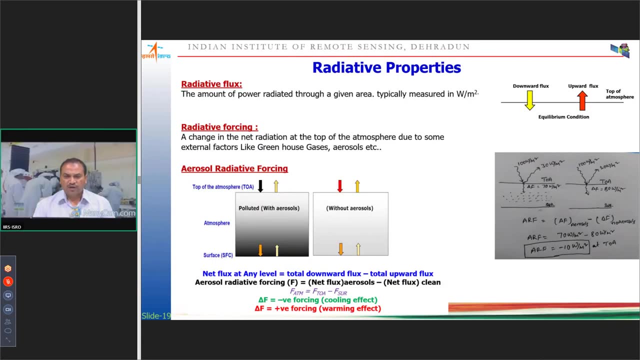 scattering or towards an absorption. but we try to understand from different optical properties and then we come to a conclusion that yes, it the inclination is towards the scattering or towards the absorption. now, in terms of the radiative properties, when it interacts with the electromagnetic radiation, so how it affects it, the the change in the net radiation flux, 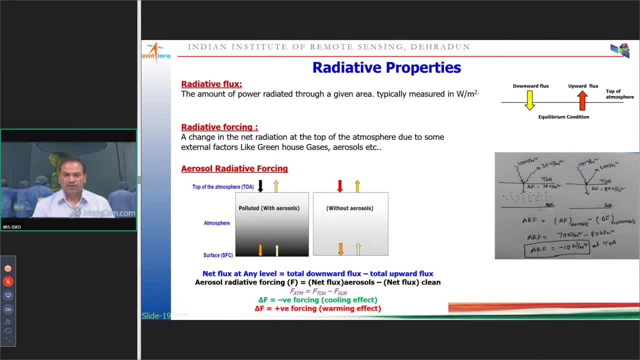 at the top of the atmosphere or at the surface. we try to estimate it. so how much amount of radiation is being received? how much radiation is scattered due to the, due to the pollution that is due to the aerosol? and suppose we there is no pollution, no aerosol? what will be the amount of the radiation that? 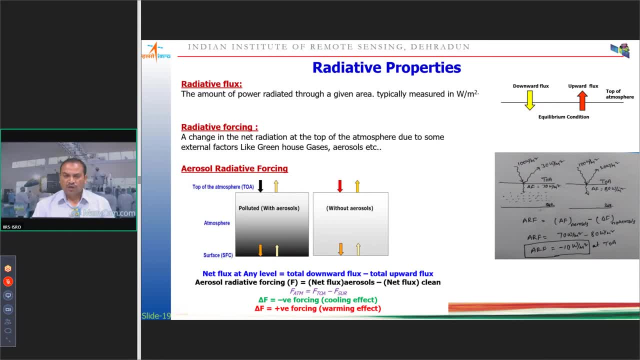 will be scattered. so we take these values, we subtract these values and then you see the downward flux and upward flux and then we calculate the net radiative forcing. so, similarly, the net flux which is due to the aerosol, it becomes the aerosol radiative forcing if the net flux is due to the 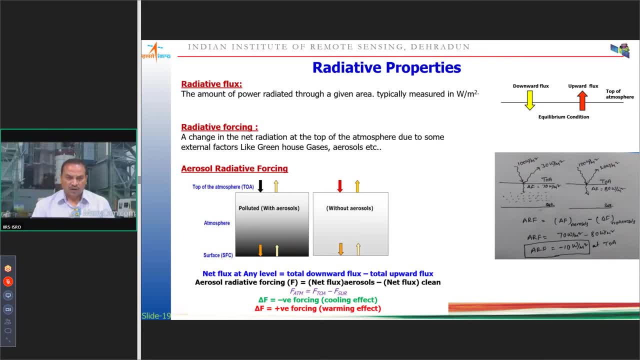 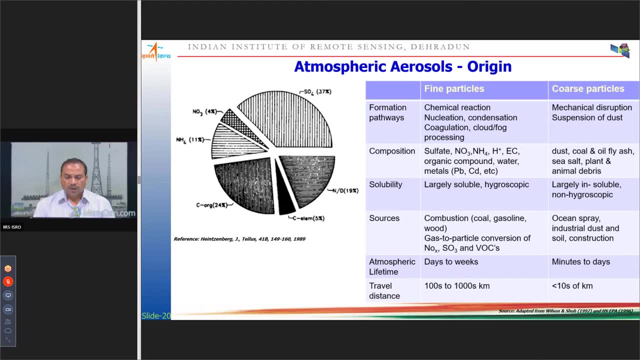 greenhouse gas. so we say that there is is the, that is, the radiative forcing due to the greenhouse gases. this gives an overview of what are the different particulates in when we talk about the fine particles or the coarse particles. so, for example, the dust, the sea salt and then the ash. these are all. 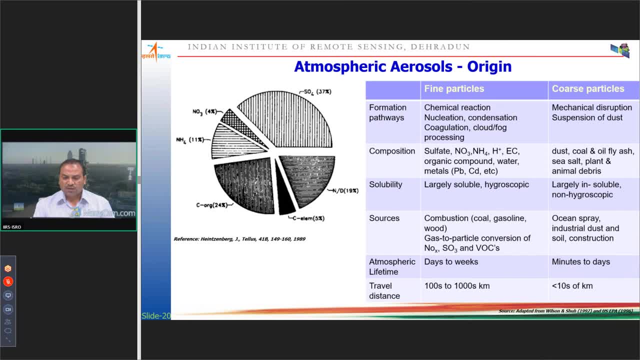 categories of these. they have coarse particles. but when we talk about the sulfate, the elemental carbon, the carbon dioxide, the carbon dioxide, the carbon or the black carbon, the, the nitrates, oxides of nitrate and nitrogen, ammonia, these are all fine particles. the fine particles are largely soluble in nature. 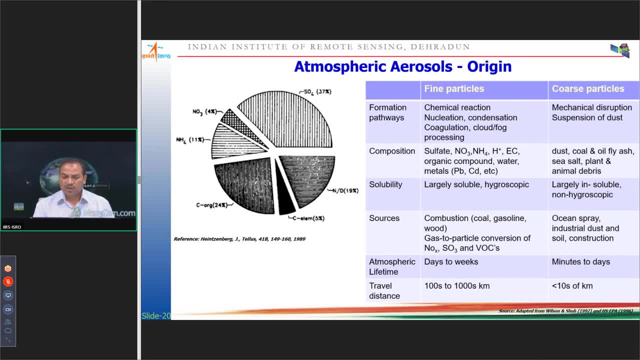 in water. but the large particles are not soluble in nature, and so when they are soluble in nature, that becomes a deadly combination for affecting pollution, the the good part of it- fine particles- is that the the resident sign is very, very small, so they are emitted and they last for few. 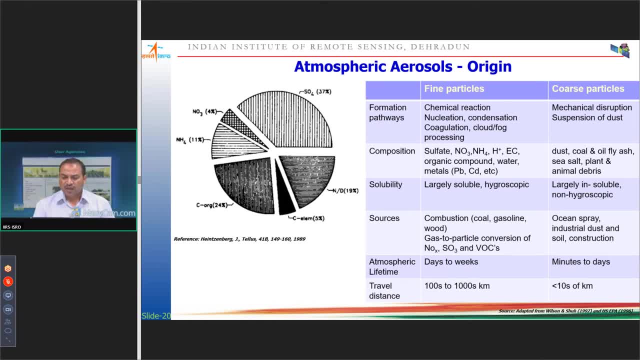 days in the atmosphere and then it decays. but the coarse particles is certain days so it goes unless and until it goes in the upper atmosphere it it settles down very easily as compared to the fine aerosols. the the biggest problem of biggest threat of the fine particles is their traveling distance. 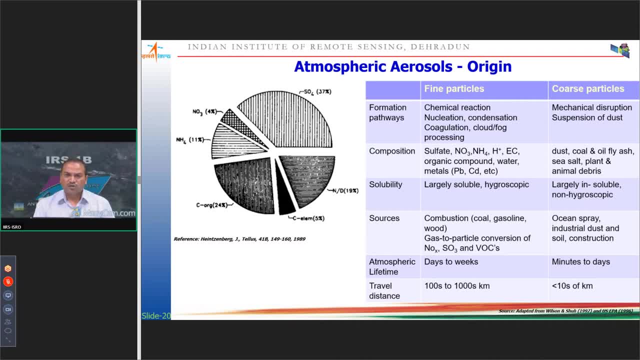 so once they are emitted from a region, the source is different, so it affects in a different region, so it travels through hundreds and thousands of kilometers and then they affect the other region as well. but as compared the course course are particles there because the heavy nature they can't stay in the 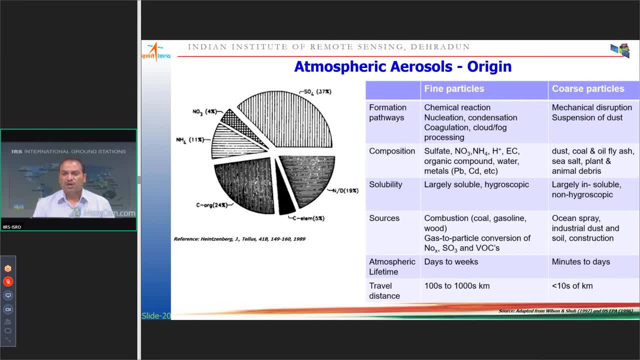 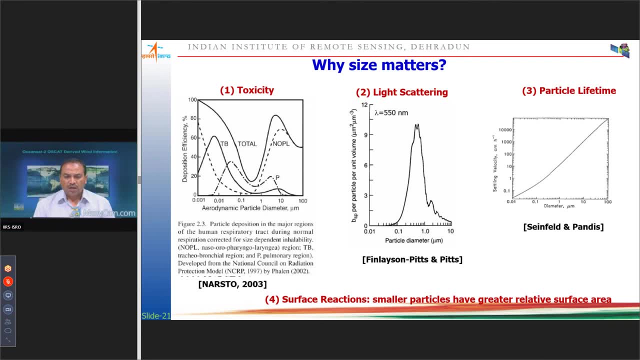 atmosphere for long. they can't go in the upper atmosphere and they settle down and they don't travel much for long distances. now another question may arise, that why the size? we are talking about size, the coarse mode or fine mode or accumulation mode, in intermediate mode, because the size has a different. 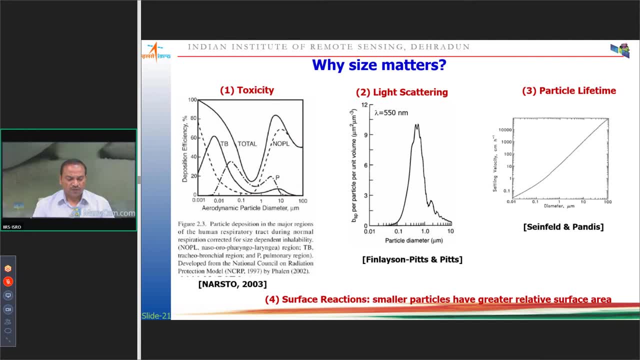 properties, the optical properties and the physical properties as well. when we talk, we have categorized into four categories. now one is the toxicity. different studies, the shows that the fine particle that is- I am talking about PM 2.5, that is all particle less than 2.5 microns they're, they penetrate in. 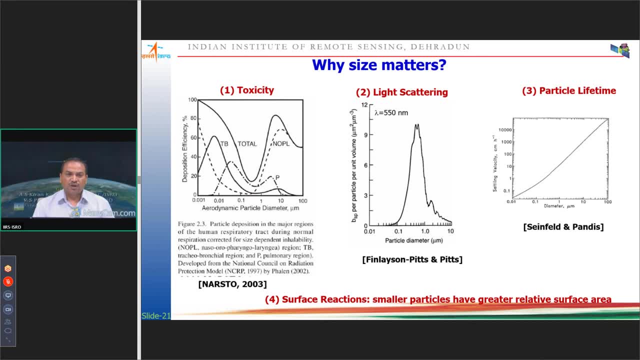 the respiratory system and they are becoming toxic in nature there. so it it becomes a problem and it creates a lot of diseases there. in terms of light scattering, the smaller is defined or is finer is the particle, more it has a scattering effect of the electromagnetic radiation. in terms of 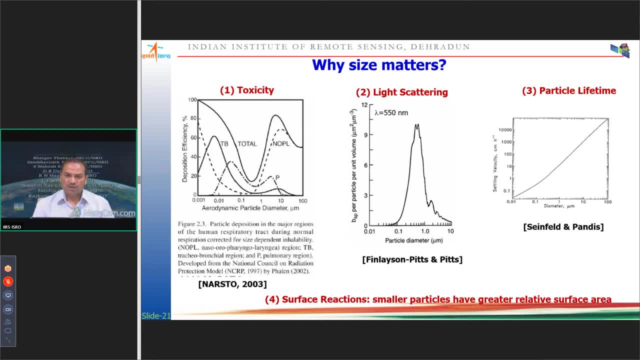 lifetime the fine particles. the more is the or less is the particle size. more more towards the fine particles, the more the lifetime it has. so lifetime becomes longer and longer. if you have a finer particle, also the surface reaction: the finer particles. you have a greater surface area so the it reacts in the 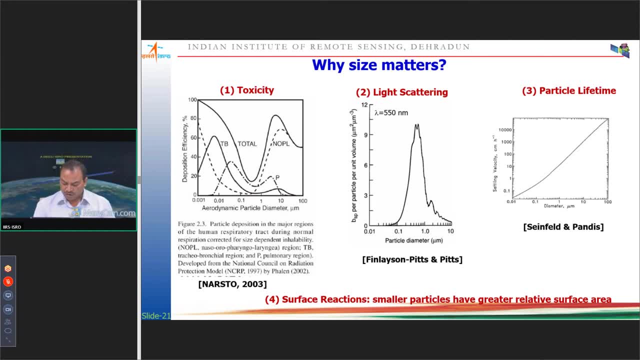 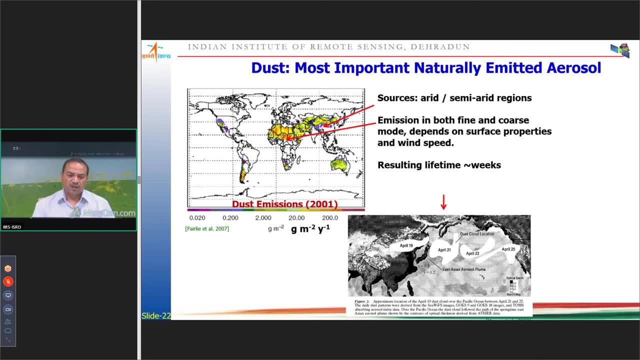 atmosphere much more reaction than the coarser particles. now. now we talk about the dust, because I said the northern African region, so these are the dominant sources of the your natural aerosols or the dust aerosols, or mineral dust aerosols. the semi-arid regions, particularly northern Africa, Middle East. 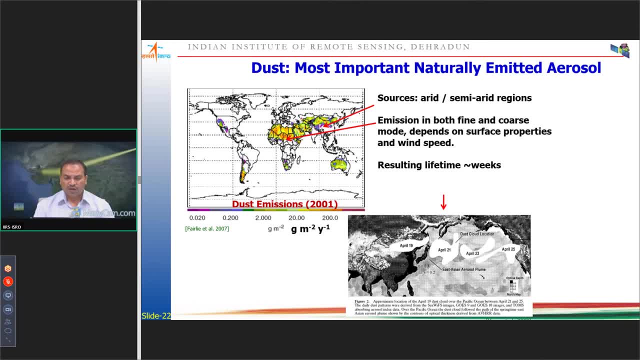 and northern China, Mongolia, northern China. they are the regions where the natural or dust aerosols are emitted and it affects the South Asia, Southeast Asia. it travels longer distances now it depends on the wind speed, wind directions, the vertical height so and it stays for longer duration because it travels to upper layers and the 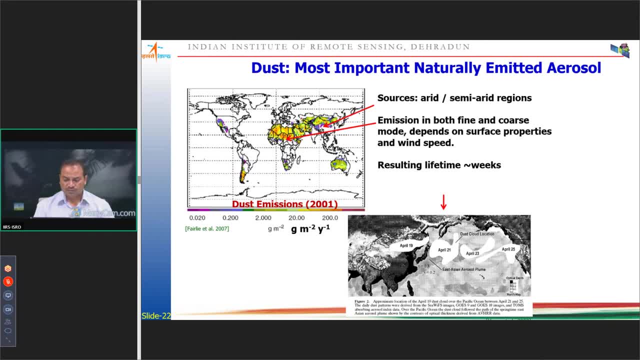 perturbations are for certain months or certain weeks now, because these particles in the upper layer, they are stable there and they are stable in the upper layer. they are stable in the upper layer and then they can react, they perturb the solar radiation and affecting for. 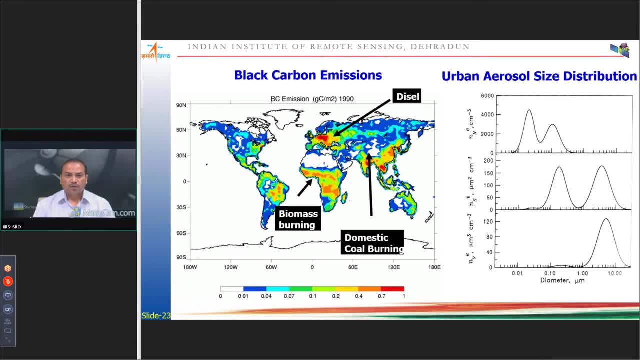 longer durations. now, if you see a region wise, the, for example, these: Asia is dominated by the pollutants from the fuel burning or the coal burning. so most of the fuel wood burning or the coal burning, so most of the fuel wood burning or the- these are the pollutants which are emitted in the most of the developing. 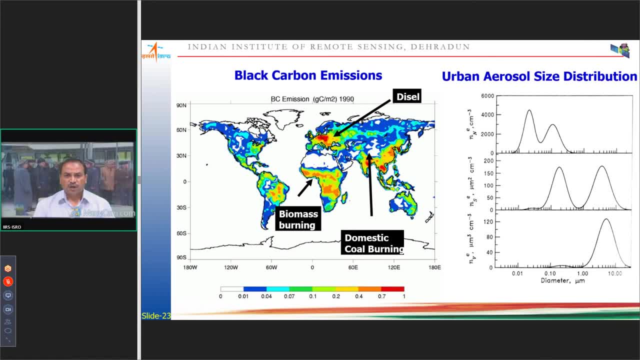 countries in the South Asia or the Asia, the diesel. most of the Europe region is dominated by the pollutants coming from the diesel engines and the African region particularly the biomass burning. so different particulates are different major pollutants or major particulates are emitted due to different emission. 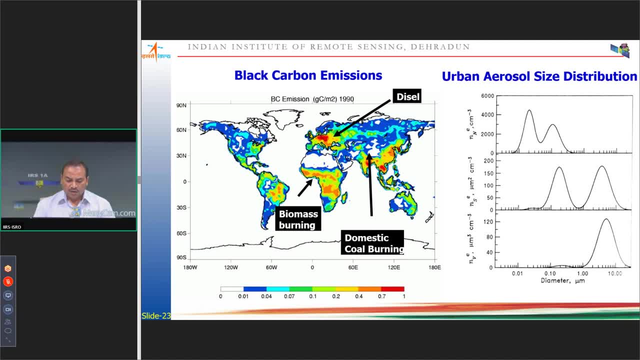 sources in different regions. then the right hand side shows the anthropogenic emissions, particularly cities. they are emitted in a finer particles, but fine particles, as I said, are emitted from the anthropogenic activities, as I said earlier. so the number size distribution shows that the number density is highest for the Fine-mode particles as compared to the coarser. 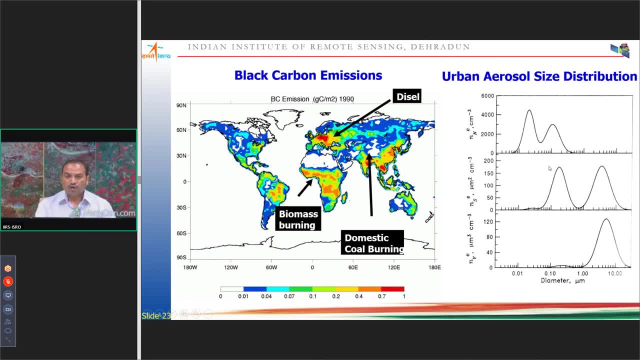 particles and these fine particles. they are emitted and from those corrosion mash into the Children's Cylinder chị, the, the carbon disposable sources of the emissions readings. the fine particles are responsible for, as I said in the previous slide, the fog, the visibility, the mist, the smoke, the smog and also the respiratory problems in the. 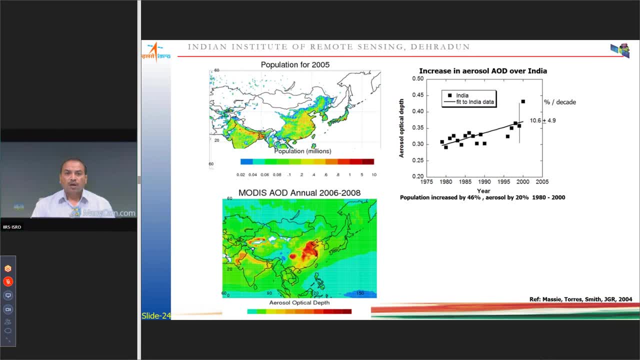 human health. this figure shows also the, the population, the. it has a direct effect on the populations of more population, more anthropogen activities and more aerosol emissions. so the figure shows that there is a direct relation between the emissions and the, or the population and the emission of on. 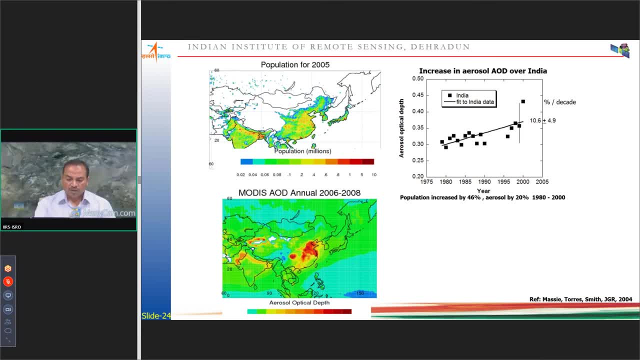 the production of the aerosols. the correlation shows that the and particularly the endokinetic plane and the South Asia is very hot spots for the aerosol emissions because the population is high and particularly what the endokinetic plane. so the analysis shows that for the 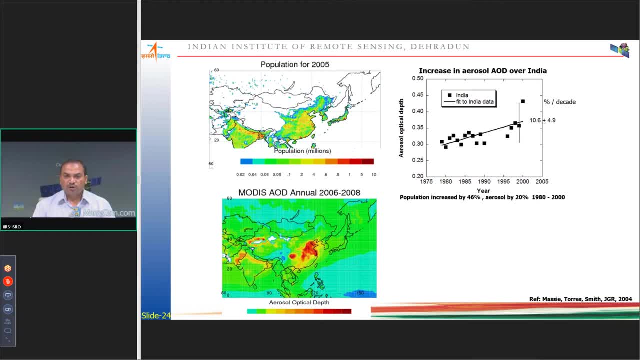 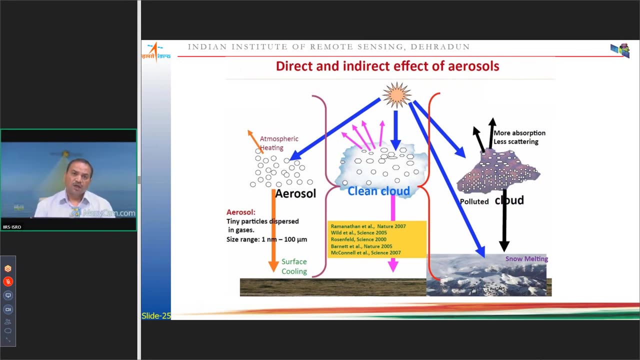 now, basically the last few years or seven, last few decades, with the increase in the population, the, the concentration of the aerosols has risen up by almost more than twenty percent. now there are directly indirect effects of aerosols. as I said, the direct effect is scattering and absorption and more of 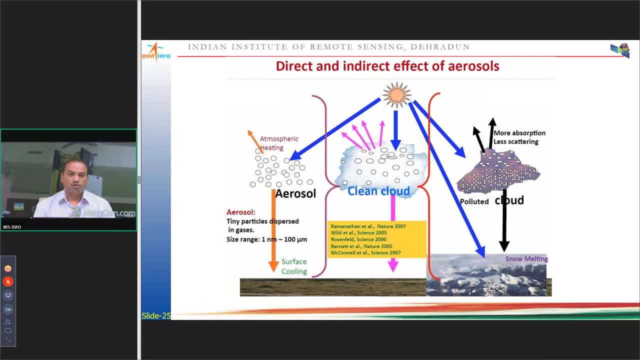 the cloud formation. now, more of the cloud formation means it is a good sign. One theory is that – one assumption that more of the – more cloud formation will have good rainfall, a good amount of rainfall. but the other – more cloud is also have a negative effect, because more cloud means less amount of radiation reaching on the ground. 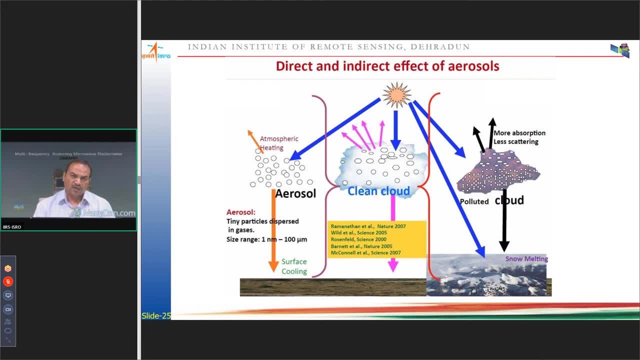 so less amount of – where there is a evapotranspiration, we have latent heat, less latent heat, so the clouds also will be less formed, and then it also decreases your rainfall. So both the combinations are there, So the aerosol will have a negative effect on the rainfall as well, as sometimes it has. 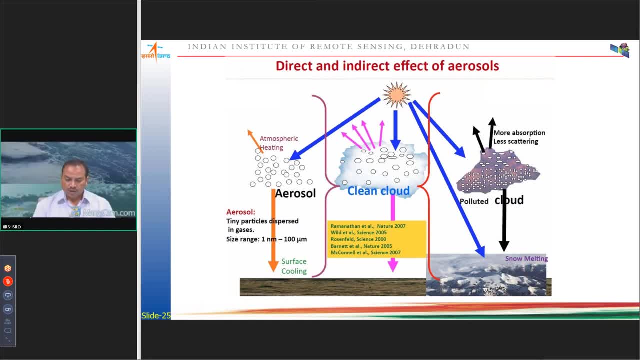 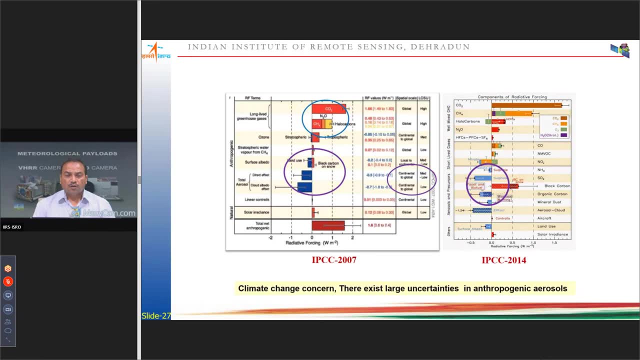 a positive effect on the rainfall. Also, if you see the – globally, it also has an effect on the climate change. Now, if you see the IPCC report, that is, the Intergovernmental Panel on Climate Change, it clearly now – it clearly comes out that the different sources of aerosol, or different 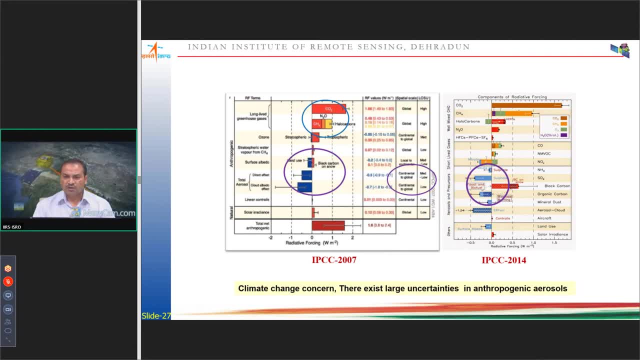 components of aerosols are having positive or negative effect on the climate, particularly the black carbon, which is having a warming nature or absorption nature is having a positive effect, so it is warming the climate or the atmosphere and the – particularly the glaciers. 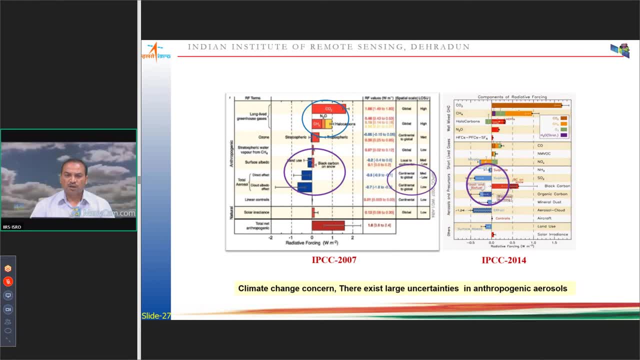 they are melting due to this warming effect They also – they are melting. So the black carbon, the elemental carbon, deposits on the glaciers, the snow, and it warms it, it absorbs the solar radiation and thereby melting of the ice and glaciers. 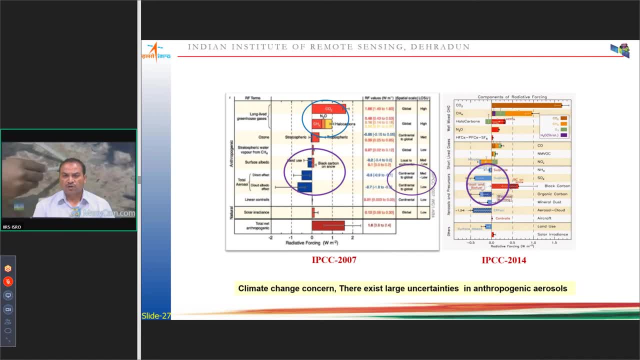 The sulphate aerosol from the volcanic eruptions – lot of sulphate aerosol. then it blocks the clouds. A lot of clouds are formed, so it blocks the solar radiation, so there is a less amount of energy reaching on the ground. 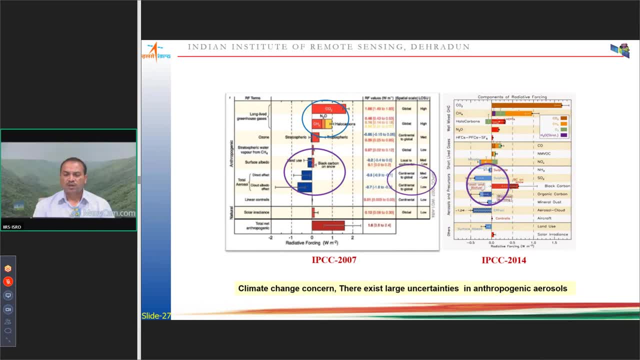 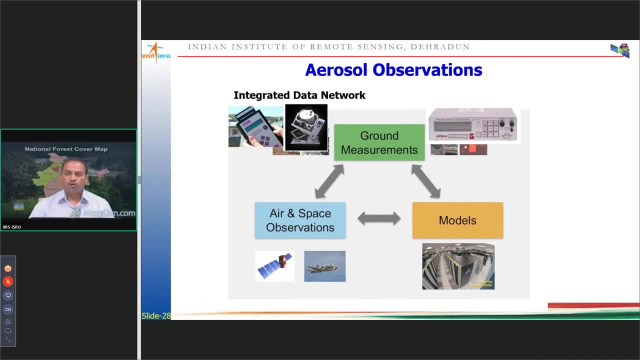 So there is a negative effect, or cooling effect that it is having on the climate. Now, how do we go for it? Because the aerosols, as I said the – we know the – exactly how we have to understand it. what are the properties? different kinds of observations we need to have. so it is. 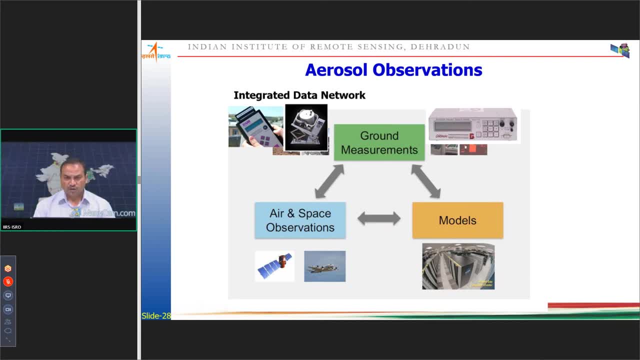 a collective and integrated process. So it is an integrated approach we have to follow. So either we have to measure on the ground and because of its highly variable nature, because tropospheric aerosol particle matter are variable in nature, so the measurement 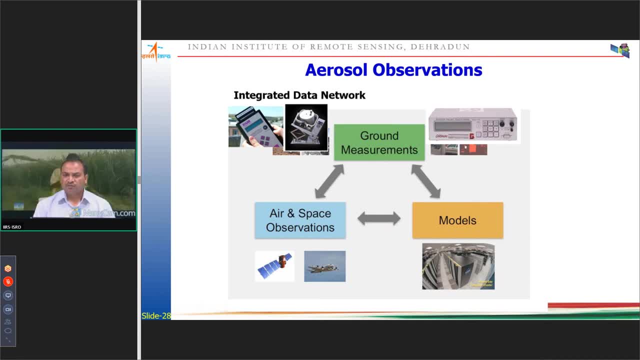 in one place cannot be extrapolated to another place. So at each and every place we have to measure, understand it, because the nature is different, the chemical composition is different, the residence time is different and the air pollutants are also different. 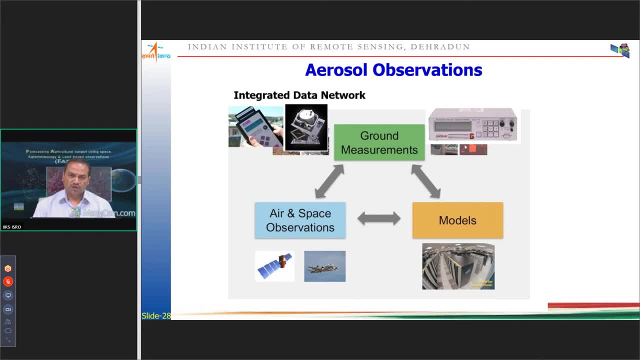 So it should be an integrated approach: The measurement on the ground with the help of instruments, Thank you. And then satellite observations are also important because it gives a synoptic view. and then there is also the importance of the models, because we need to understand it. and then 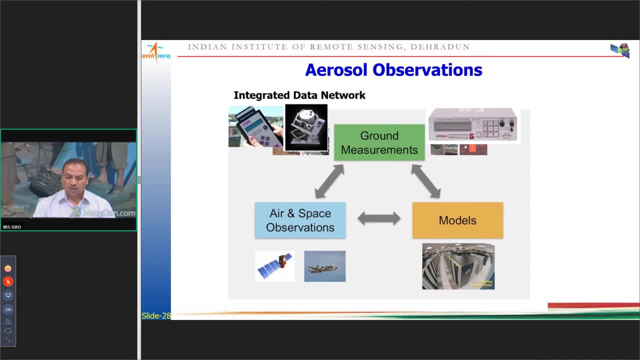 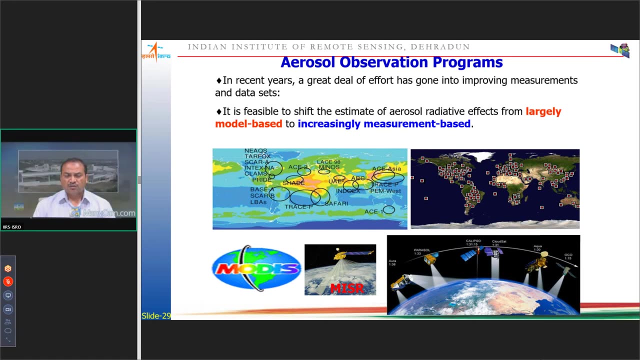 we can use these simulations for forecasting it. So this collective approach will help to understand and to study the aerosols. Over the years, there have been different campaigns. There have been different campaigns to understand it, whether it is the sea campaigns or it is. 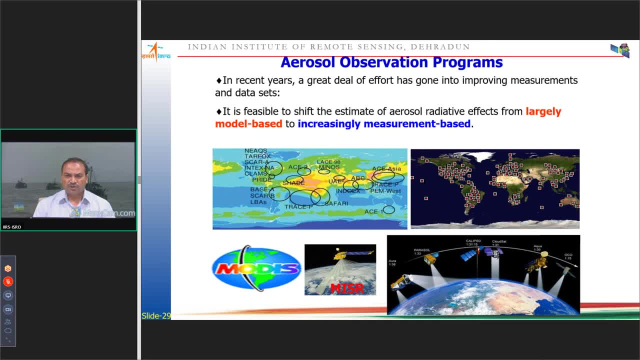 a land campaign. So different countries, different regions adopt this scheme and they measure with different instruments, take to the different oceans, cruises, or in the land and they come out, And there are certain permanent stations over the land which is done by different parts. 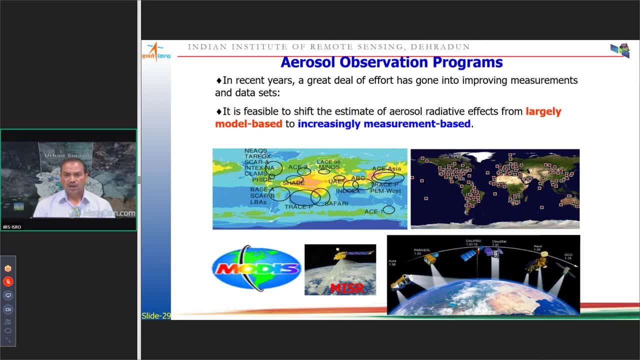 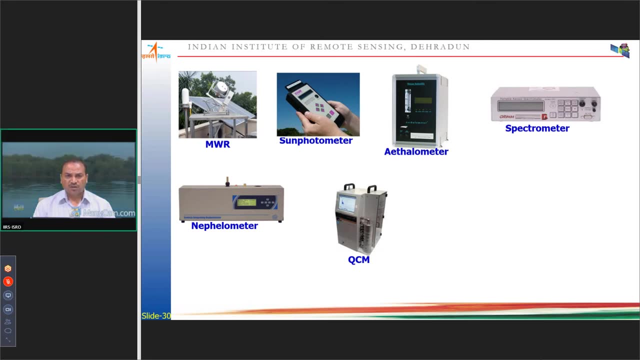 of the countries in different continents, Like India. India has its own network of instrumentations and they measure it continuously over the ground on different parameters. Now, some of the instrumentations which I a glimpse of it, I will give here. One is the top left is the MWR, that is, multi-wavelength solar radiometer which has been developed. 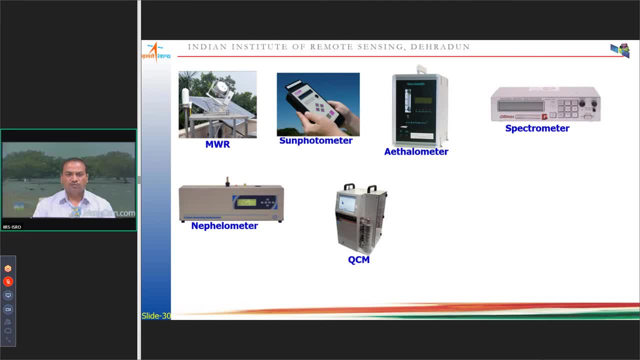 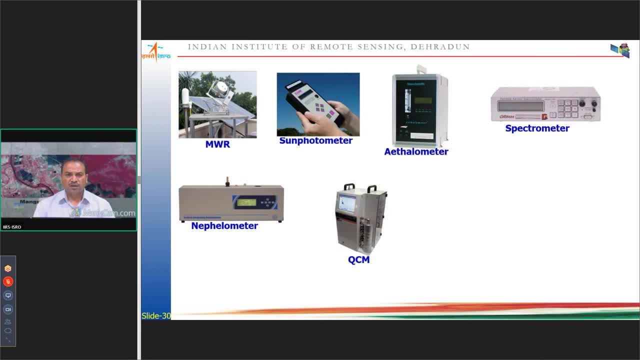 It has a 10-channel wavelength, from ultraviolet to near infrared. So it measures solar radiation and then it different physical concepts, physical equations. it calculates the optical depth at different wavelengths. It measures the aerosol optical depth. So what is the? what is the extension coefficient? 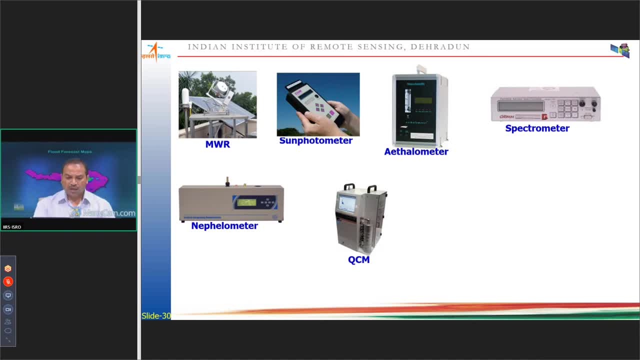 That is the degree of the pollution. And the another instrument is a sun photometer is a five wavelength instrument which has different filters. It measures ultraviolet to again the near infrared And another instrument is the ethylometer. 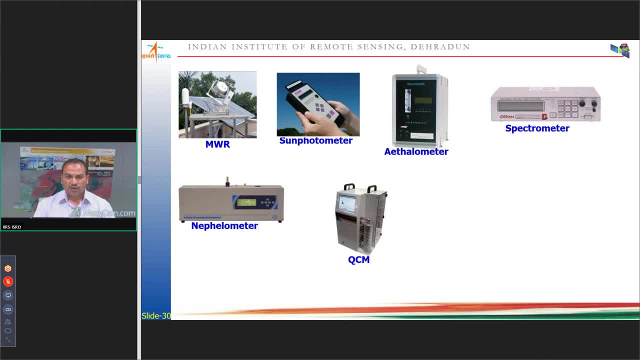 The ethylometer measures your black carbon or elemental carbon in the in the aerosol. The spectroradiometer it measures the aerosol mass and the particular- sorry, the aerosol mass concentration and particular number density in a in a column. 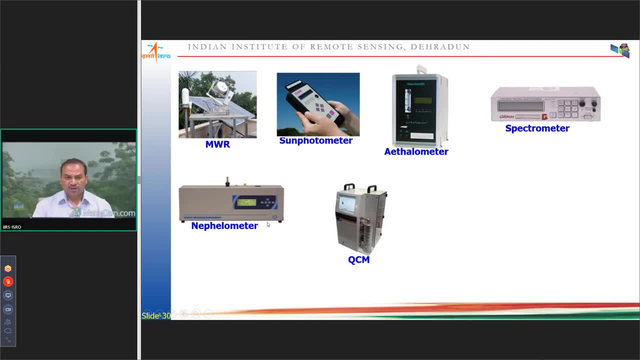 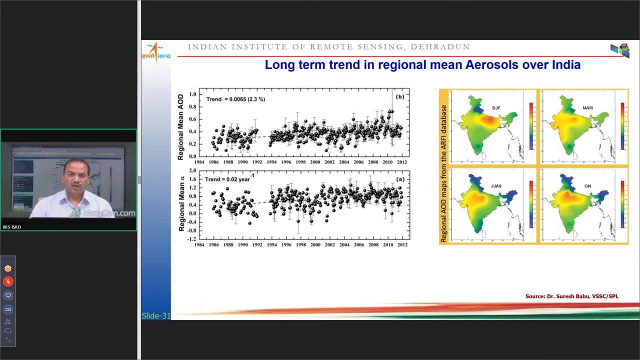 The nephelometer measures your scattering coefficient. it gives the information on the scattering coefficient, And the quartz crystal microbalance QCM measures your mass, the number, concentration, the particular, the particular size, distribution and so on. With the help of these integrated approach, you can measure the long-term trends and long-term 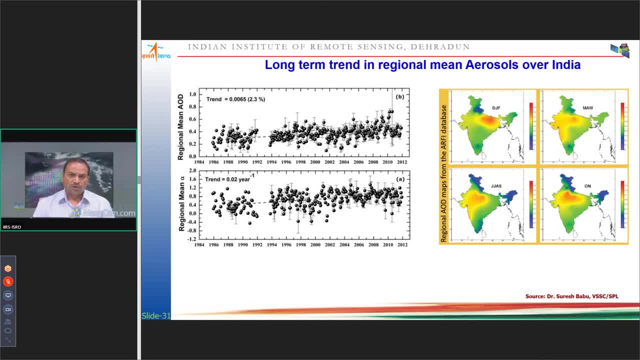 effects And of the aerosols, and particularly, for example, the last three decades. this is the scenario: A continuous monitoring stations all over India, different regions, different cities of India, And this is the trend of in the last three decades, how it moves, though it is increasing. 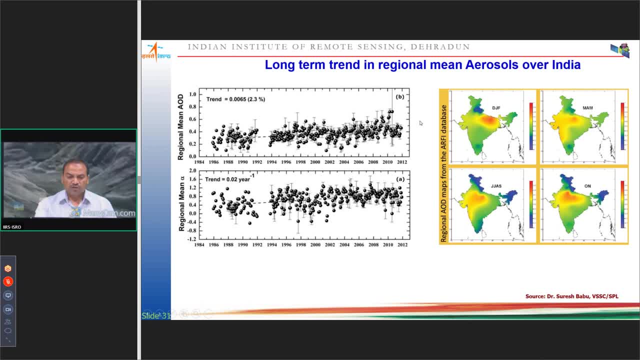 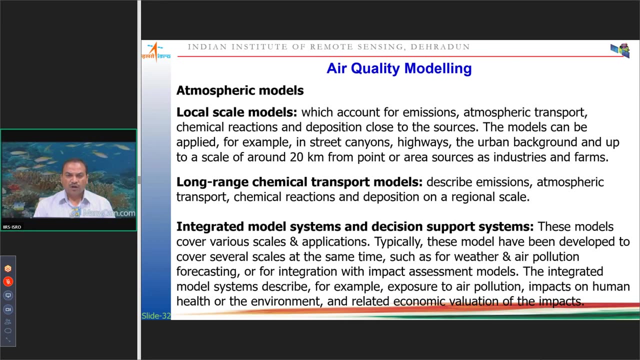 So aerosol optical depth- and this is exponent- It has been increasing due to the anthropogenic activities And overall the synoptic picture We can get in the form of a map from the satellite data as well. Now the you can have the air quality modeling also. 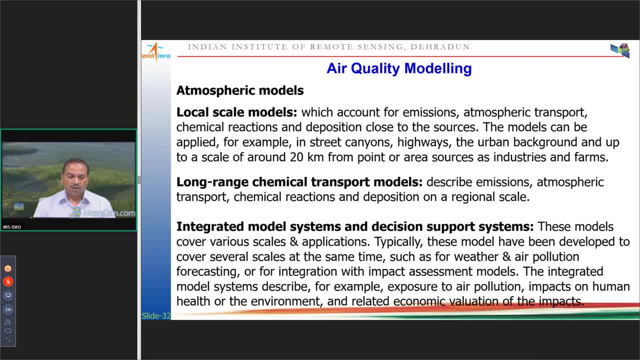 So the broadly the models are distributed in a local form, like local scale models, So it accounts for the like street models for a small city, So street canine models. so you take the urban background, the ambient background and then 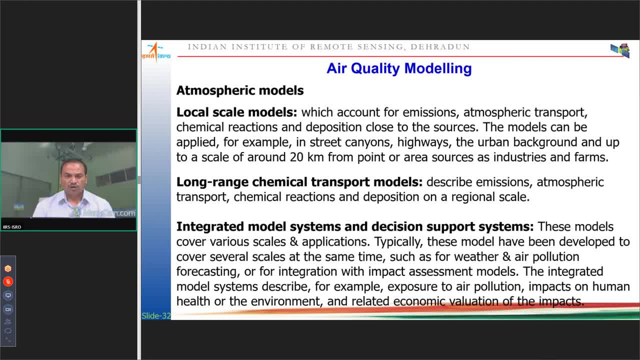 it tries to Understand through the local metrology, the geometry of the lanes, the buildings and the vehicular traffic density and all that And the and then the vehicle efficiency, because a different vehicle have a different engine efficiency. 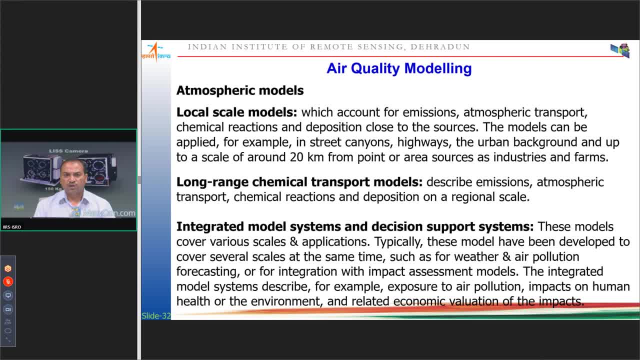 So all put together then it scales around 20 kilometers from the point source And then it tries to understand the local, the emission inventory. The second class is long-term, Long-range chemical transport models, So it describes the emission, the atmospheric transport, the chemical reactions and the 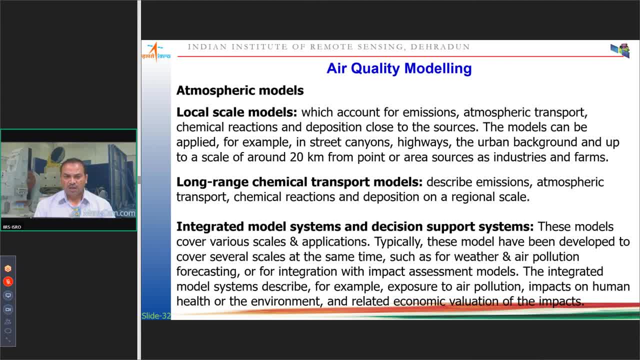 deposition on the regional scale. The another approach of the atmospheric model is the integrated model system, where it forms the integrated approach and also comes with a decision support model. So these models cover various scales and applications. These have been developed, Yeah. 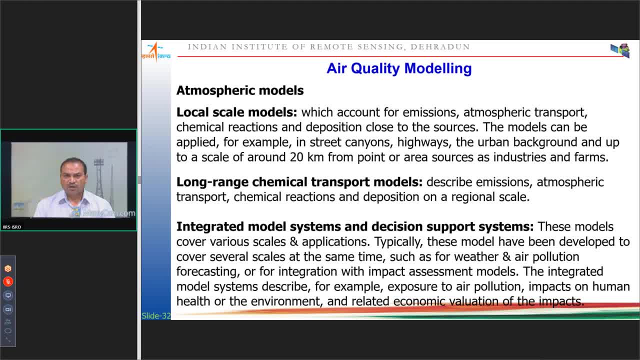 For the air pollution and for the weather studies and also for the forecasting of these. So it is the integrated system. So in this this can be used for all sorts of the understanding and the air pollution, the environment and the impact on these, of the air pollution on the environment. 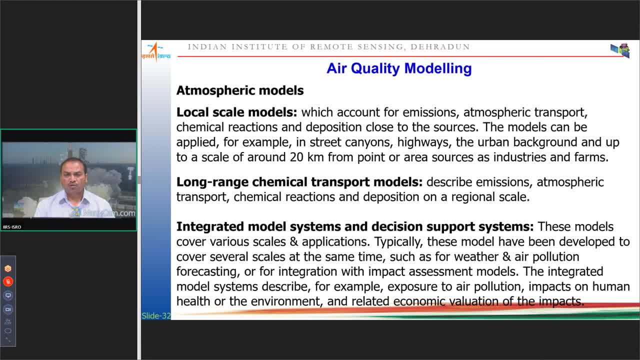 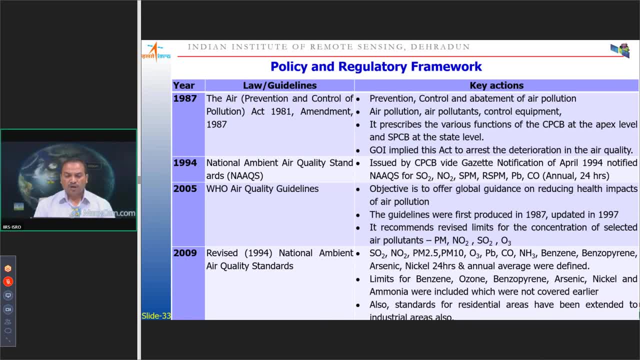 And this has a from low level, So local scale, to regional scales Now as India is concerned. so we had tried to understand and for keep on from decades together this has come notice of the policy maker and from time to time there has been 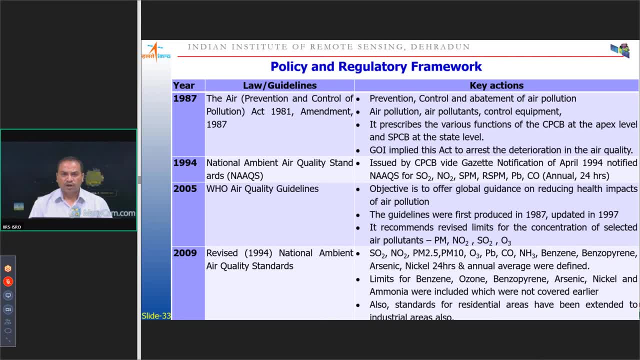 many acts, many policies which government of India has adopted And, to name a few, the Air Prevention and Control Pollution Act of 1981. It's a very famous act and which was amendment 1987. So it gives here the prevention, control and appatment of the air pollution. 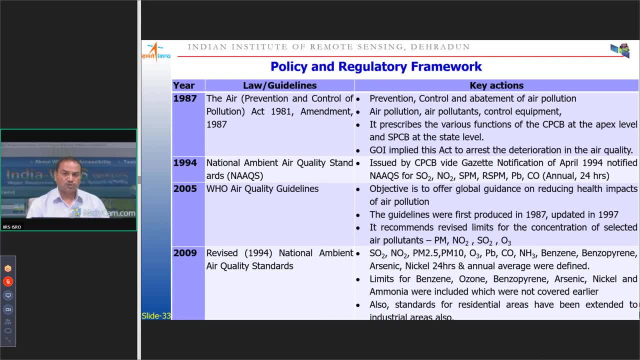 So how to decrease it, Not only the prevention, the control, but of all, what are the steps to be taken to decrease the air pollution or to make the cleaner air towards the cleaner air? So it talks about the air pollution, the pollutants, the definition of the air pollutants, what. 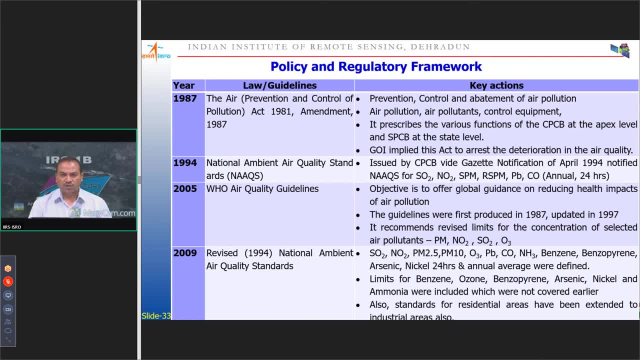 are the different pollutants and the control equipments, whether it is the society or the industries. So what are the different equipments and what are the? and if these are not in control, what are the implications or what are the penalty to be imposed on it? 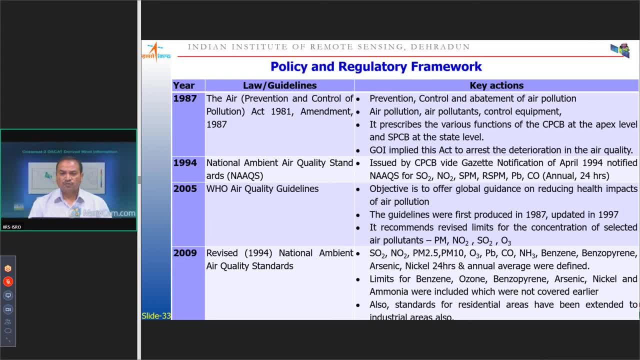 They also in this act they prescribed the formation and the functional of the central agency of the pollution board, the CPCB Central Pollution Control Board, and also at the state level, the State Pollution Control Board. So these are the APECs, CPCB, APECs at the central level and which is supported by the 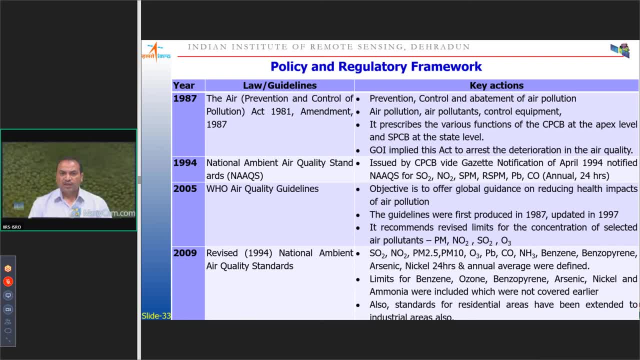 Pollution Control Board at the state level And 1994, the Government of India came out with a National Ambient Air Quality Standards for different pollutants and which was appended or added in revised amendment in 2009 of the NAQ standards. So in this the particulate matter, SO2, the CO ozone, and also added with the benzene. 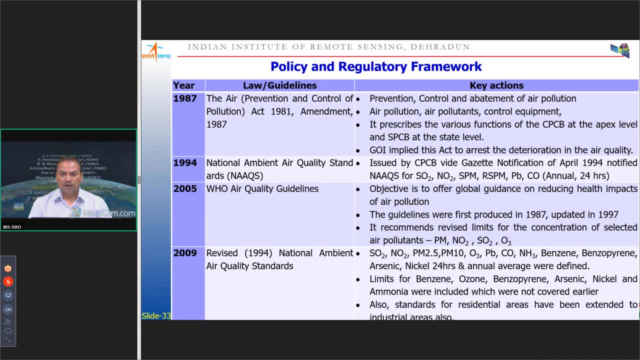 the ammonia and so on, the arsenic, nickel and other things. So there is a standard given there for different air pollutants and different areas, whether it is a residential area, rural area or industrial area. So all abbreviations are given here. 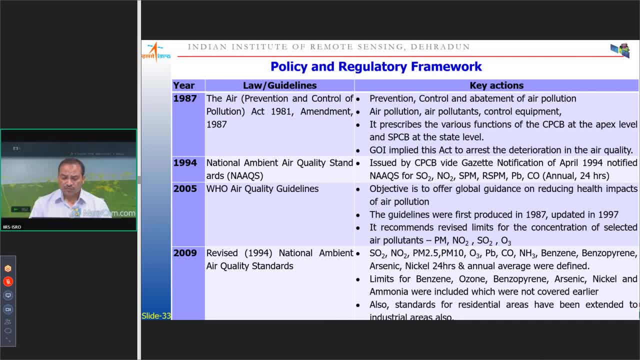 Thank you. Apart from these, the Government of India also had put into record the Motor Vehicle Act of 1988, where it is a must that the fitness certificate of the transport vehicles has to be produced. So every the rider has to produce the fitness certificate and 15 years of vehicles diesel. 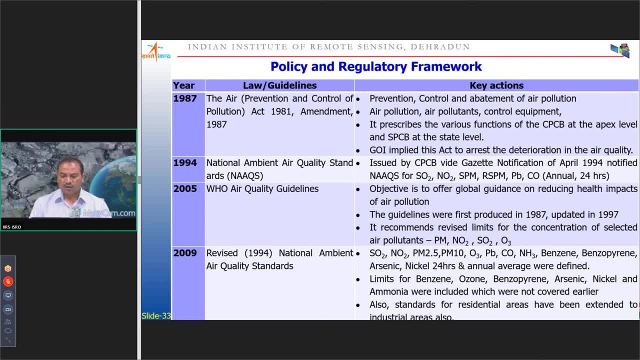 vehicles and other things have a proper procedure wherein these, every vehicle has to have a fitness certificate. Every engine, every vehicle has to give the fitness certificate. Then this 1988 Motor Vehicle Act was amended in 2017.. This is an amendment in 2017, that every that the certificate has to be – they were 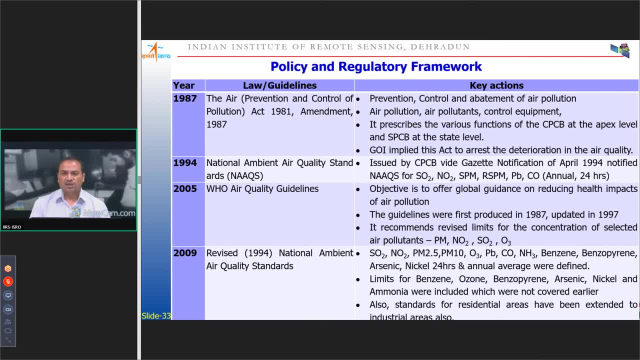 nomenclature that the certificate has to be produced by a concern agency. They have identified a concern agency and recognized the concern agency and those agencies have to give the certificate of the vehicles fitted. certificate of the vehicles. Okay, Okay, Okay. 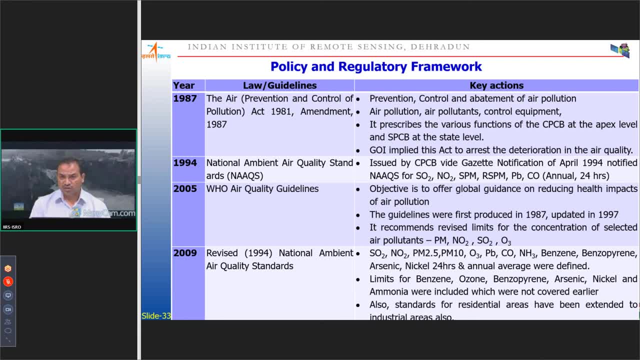 And this will be done with the automatic testing machines. So the certificate will be issued by automatic machines And the first October 2019 it will be implemented. So all the vehicles apart from now, Bharat standard 6 also will be coming in 2020.. 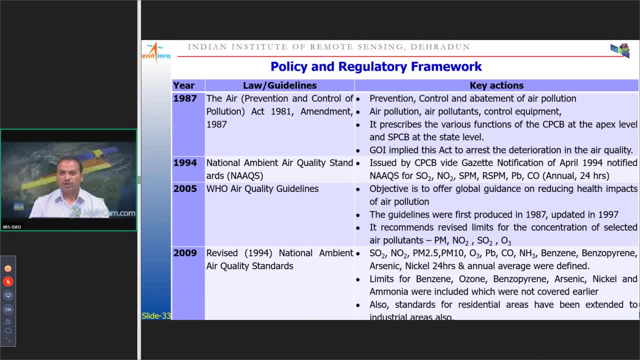 And then the regulations of the air pollutants will be under control, Because there are different, higher standards given to control most of these air pollutants, like non-methyl hydrocarbons, carbon monoxide, particulate matter, NOx. So very high standards are maintained in the Bharat standard 6.. 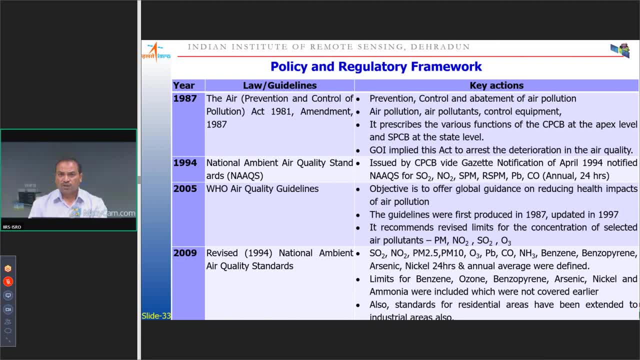 Then also the government is also focusing on the use of the e-vehicles, like e-vehicles, two wheelers, Three wheelers, the metros. now many cities have metros, which is, non-fossil fuel based engines, And also the government intends to have from 2022, the two wheelers with 150 cc, all electronics. 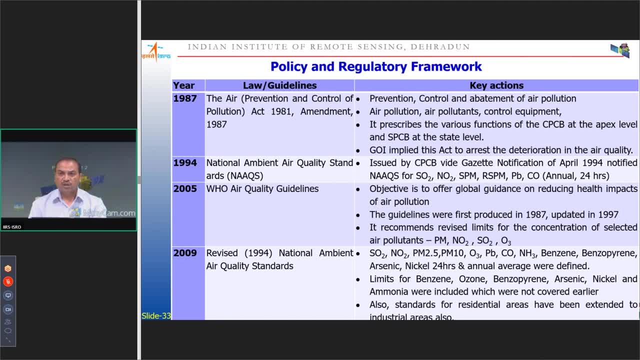 two wheelers And by 2023 the e-three wheelers, And by 2023 the two wheelers will be available in the country, and also promotion of the electric cars. Also, India is signatory of the Paris protocol, wherein India is committed to reduce the emissions. 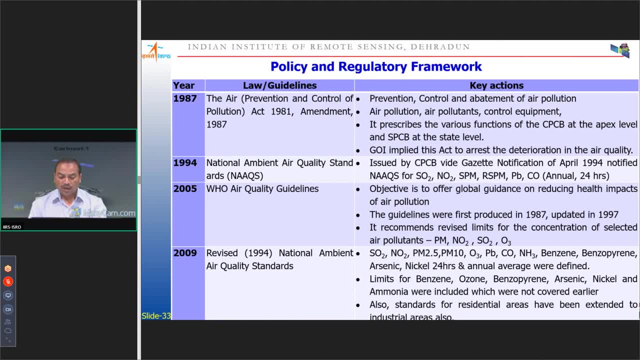 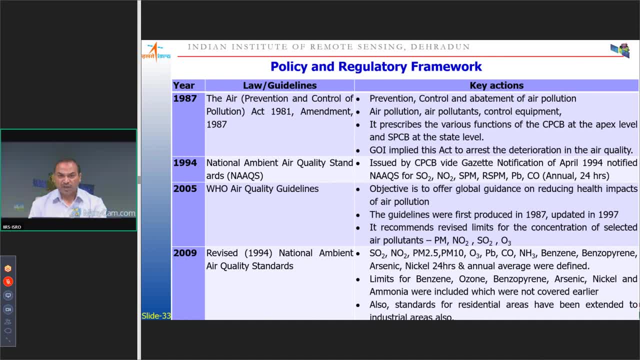 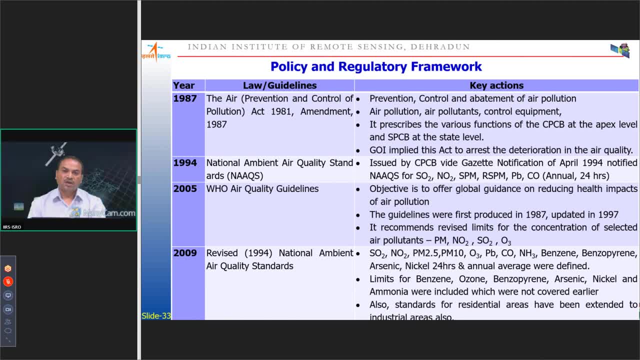 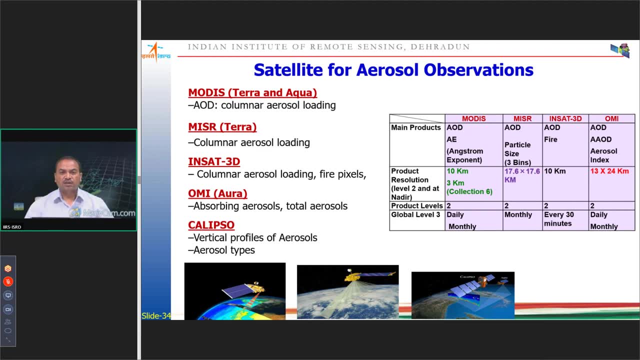 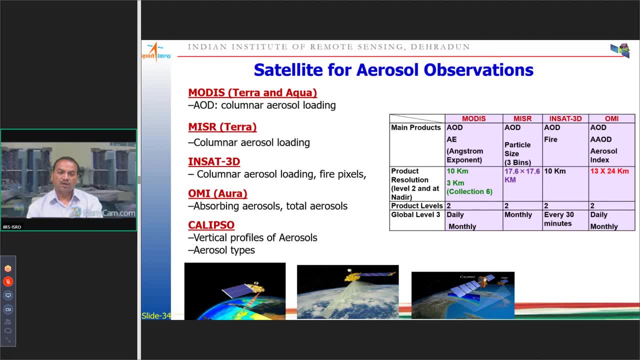